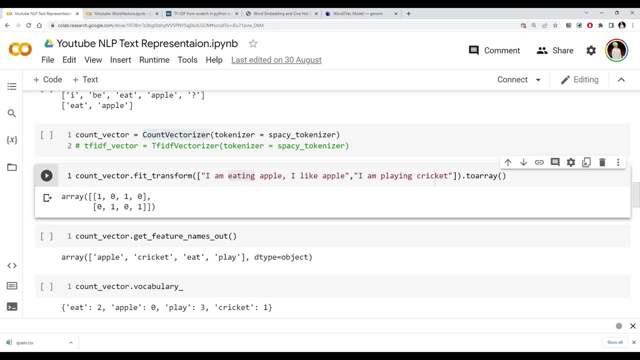 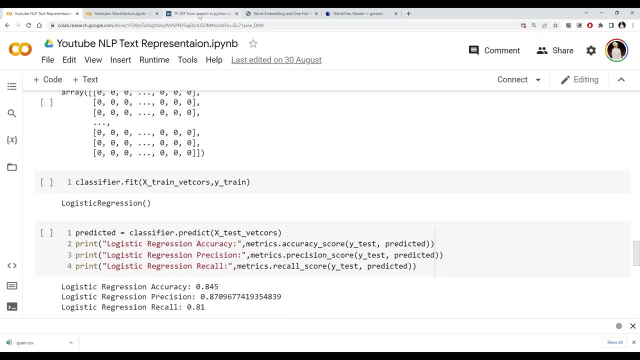 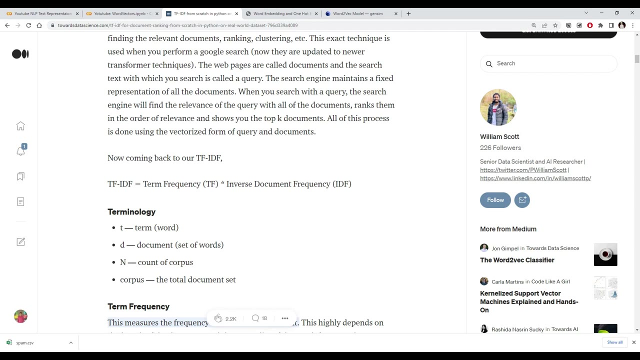 And the next technique we saw was the TFIDF technique, which is somewhat theoretically better than what we have in a count vectorizer, because in TFIDF we calculate score for each word, and that code, that particular score is, depend on these two things. 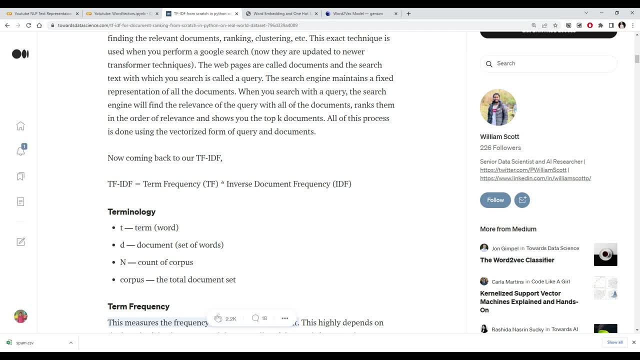 The first one is the term frequency and the second one is the inverse document frequency. So the term frequency is nothing but how many times that particular word has occurred in that sentence, And inverse document frequency is nothing but how rare that particular word across the other documents. 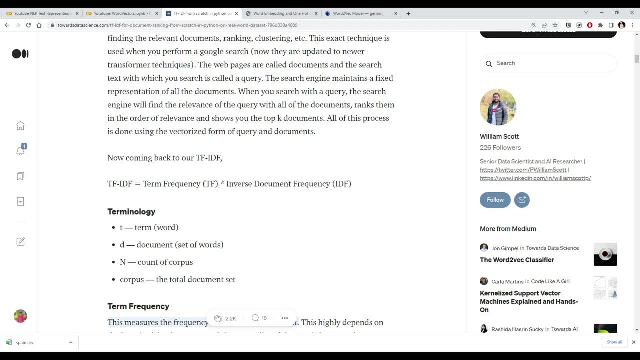 So if you have a word which occurring very frequently in that particular document but it occurs very rarely or not occurring in the other document, then that particular word will get high importance for high TFIDF value. So that was the second feature: engineering technique. 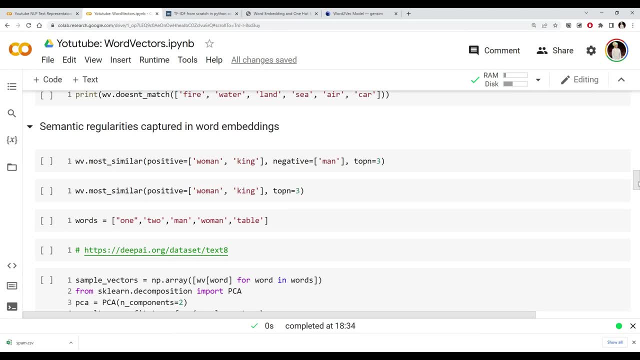 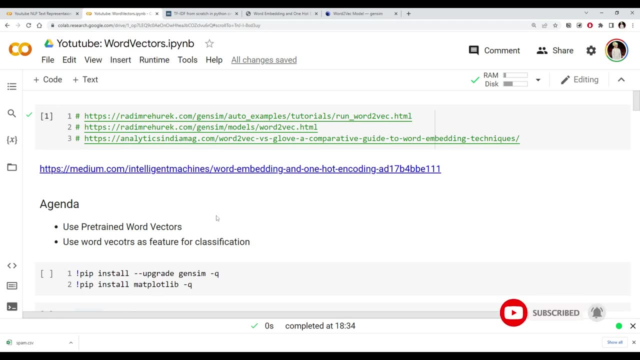 Today we're going to look at the third one, which is nothing but the word vector. So you might have heard of word2vec thing, right? So that's what we're going to see today. So we will see How to use the pre-trained word vectors. 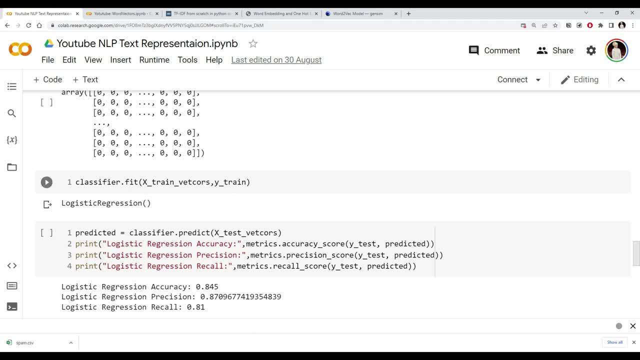 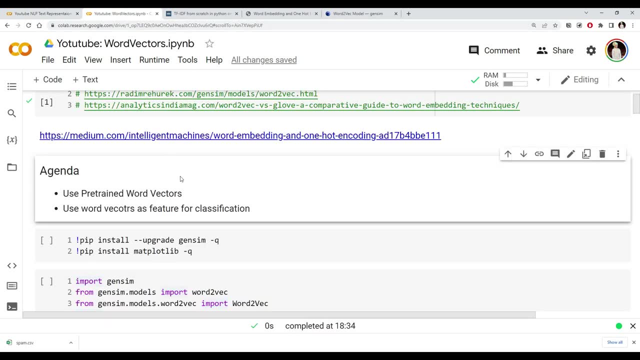 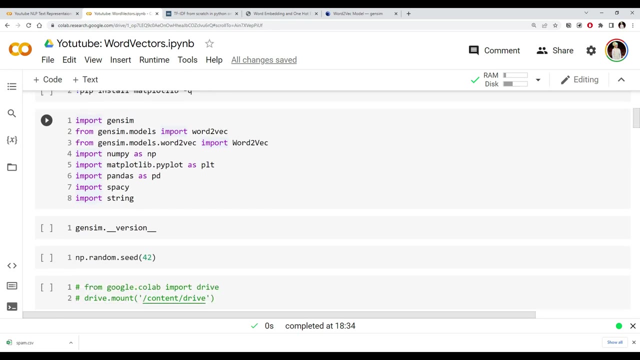 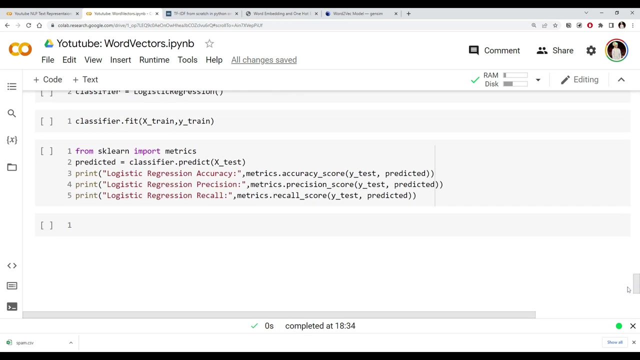 which is nothing, but you still have a vector representation for your words And we will see how to use that particular pre-trained model, use that pretend model to calculate the vector representation for our dataset And then finally fit that particular feature vector representation for the machine learning model. 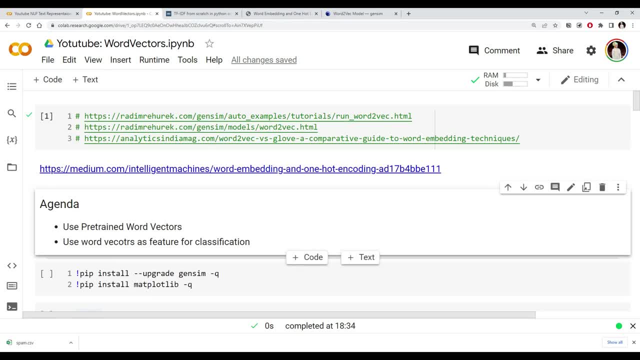 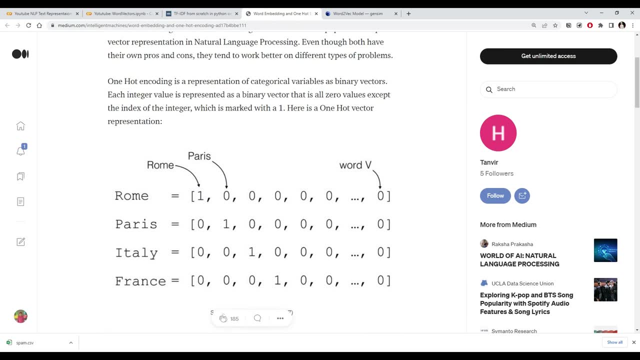 we will see whether we get better performance or not. right, so what exactly you know? word vectors or what to act. if you look at the, you know how do we represent a particular word. so one of the thing to represent a word is called one. hot encoding is nothing but what we first do. we. 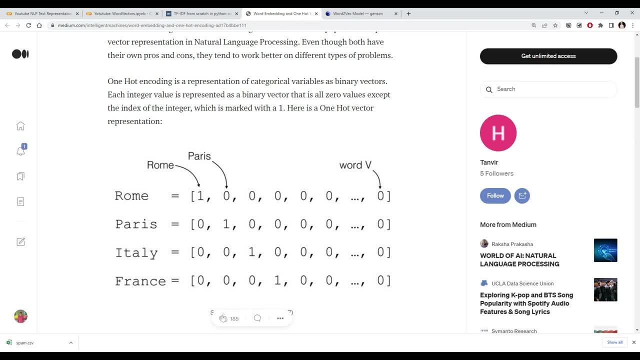 find out all the unique word in your data set. let's say we have a 10 000 unique words in our data set. and then what we do? we assign a unique index to each word. let's say, you see this word room. we assign index one. let's say there is another word- paris- in our data set. we will assign. 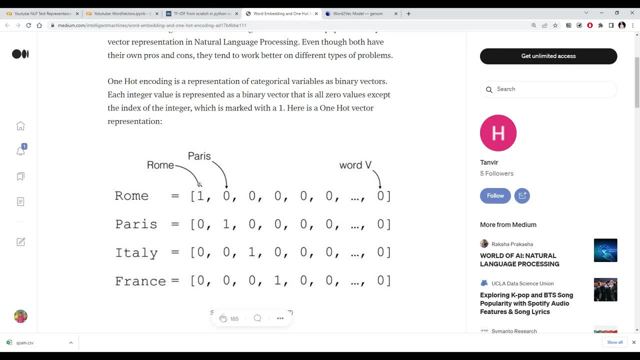 it index, let's say this particular, the first index. this is the zeroth index and, similarly, you will have index for each word, and then if i want to represent this particular word, rome, then what i will do? i will take one vector right of a length equal to the number of 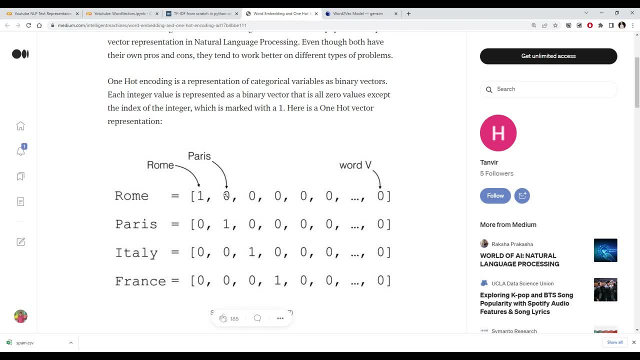 of unique words i have. so this will be of length, 10 000 dimension. and then what i will do? i will find the index of the room, let's say, which is the zeroth index, and i will put one there and all other values will be zero. this is how we represent particular word room. similarly, for paris. what 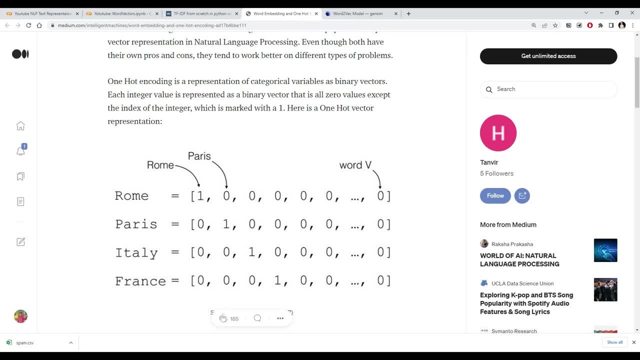 we will do. we will find the index of the paris in that 10 000 dimensional vector and we will put one there. but the problem with this representation, when we represent row or this paris using this long vector, the first thing is this vector representation is very long, right? so first, 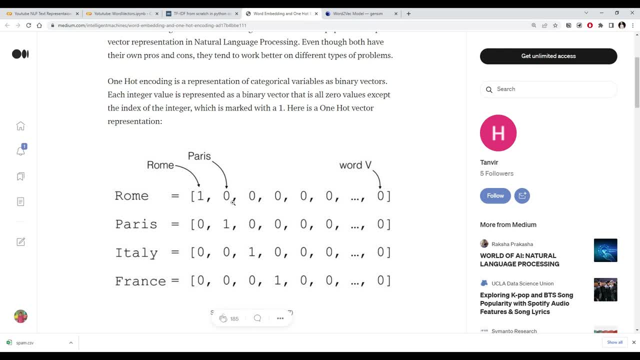 of all, if you have 10 000 words- so let's say you have one lakh words- then each word needs to be represented by that one lakh vector. right, and then you will see that this representation is, most of the things, will be zero, so it will be a sparse matrix or that particular sparse vector. 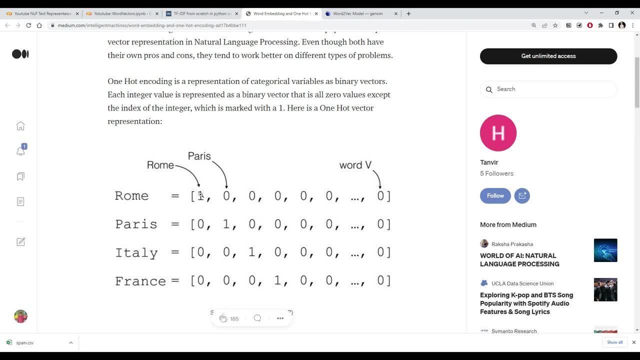 the second thing is we are not able to compare the two words. so mathematically, if i take the dot product of two numbers, that tells me how similar these two particular vectors. so if i have a words, we let's say i have three words. two of them are more similar to each other and one of 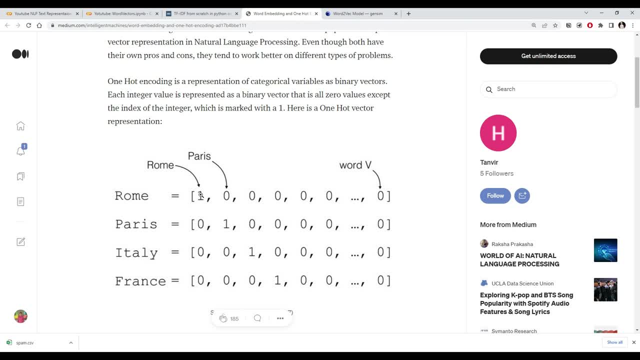 them is, let's say, dissimilar to them. but if i take the one not encoding, no matter which word dot product i take, with which vector, the dot product will be zero. so even though you can see that, let's say there is a paris and the france which are related to each other, their dot product will be. 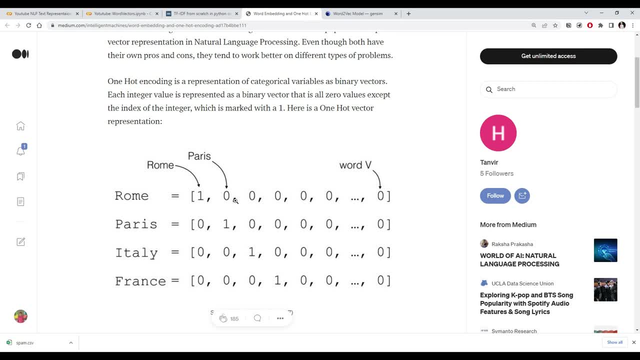 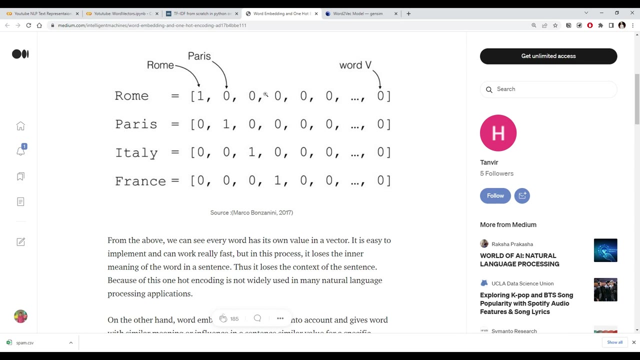 the zero. so this is not a good representation. when we want to compare certain words, whether we want to, you know, have this meaningful vector representation- and that is where the word vectors comes into the picture- then how do we find such a vector representation, which will be comparatively? 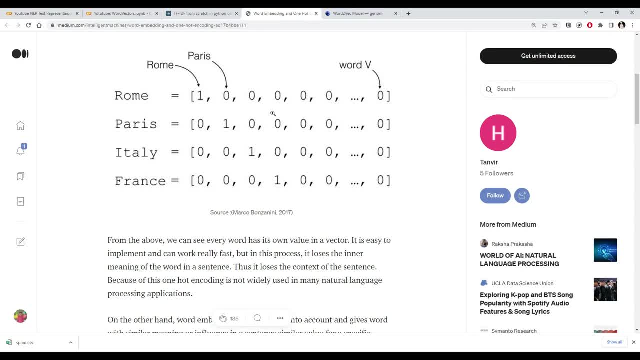 you know, you know less number of vector size, or you know smaller vector size. instead of having this ten thousand dimensional, we might have, let's say, 100 dimensional or 300 dimensional vector, and also we should be able to compare the two vectors. right? so that is overall intuition behind the. you know the word. 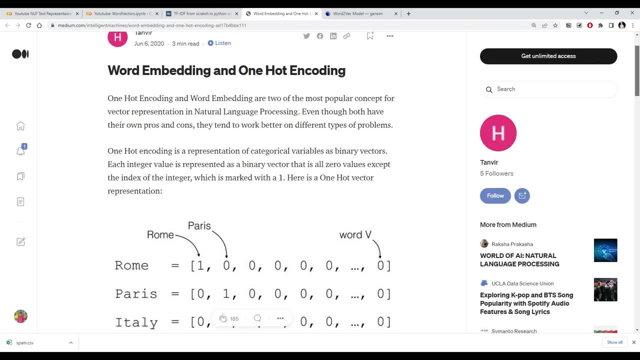 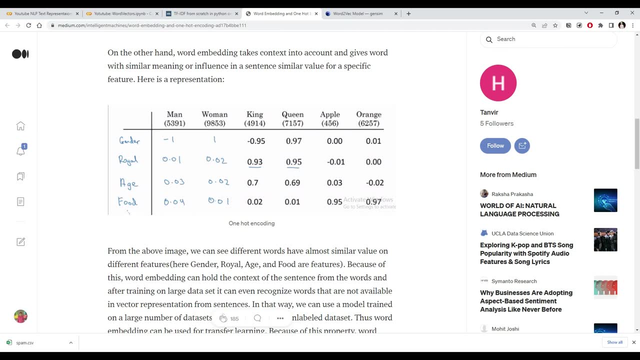 vectors. so here is the, this particular block. right, they have given a good intuition here, so let's think of that. we decided to create a vector of dimensional four to represent each word with the four dimensional, and we can intuitively think that that, let's say, one of the dimension represent. 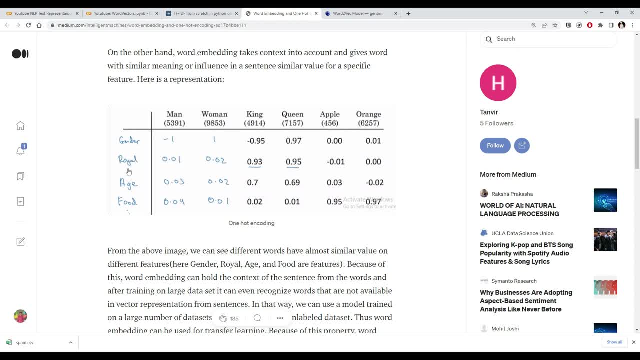 the gender aspect. the other represent the royalness aspect. now, this is something we are thinking right. it need not to be the same. but then what happens? if we have some meaning for each dimension of the vector, then depends on the which word we are representing. those values will change. for example, 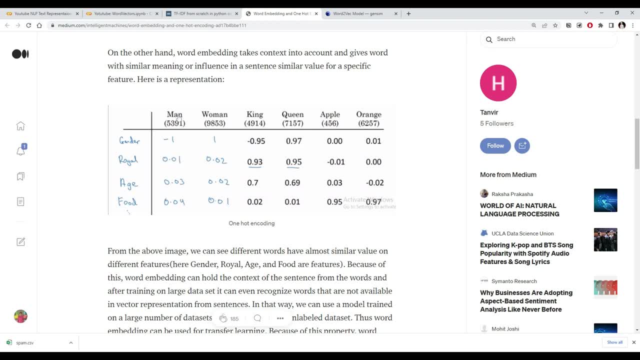 if you look at this particular vector, let's say man, so the man will have some high value for gender, but it might not have some value for, let's say, royal or the age or the food, because man is more of like in gender. similarly, for women we will have high value for the gender and the for other dimension. 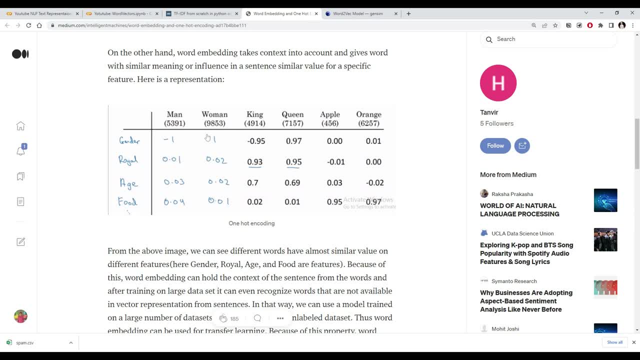 there will be a smaller value and again you could see there should be some difference between those two values which represent the gender for both men and women. similarly, if you look at the king, definitely the king has two aspects. first of all, the gender is towards the man. 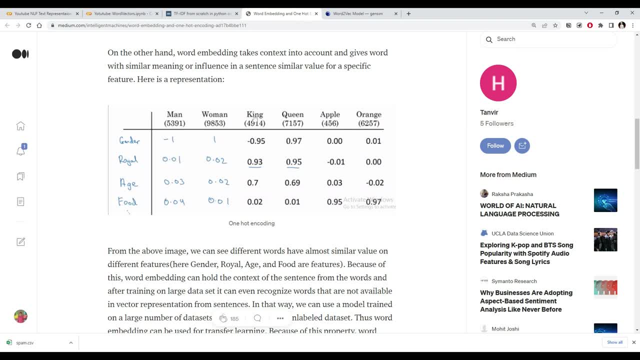 so it should have high value for gender and it will also have some value for royalness, which was not here, right? so this meaning you should be able to see if you are able to represent these words using the vector representation, whose dimension actually encodes a meaning. 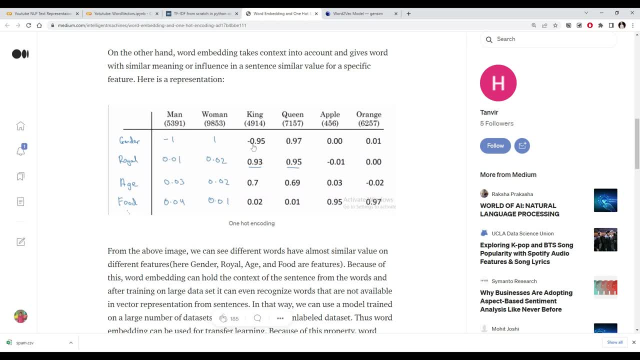 because of this thing, what will happen? you should be able to compare the vectors of man, or vectors of king, or vectors of women and queen, and even you can perform some arithmetic operation. so that is the intuition. i'm not going too much into the theory because my focus will be on hands-on thing. we will see how to. 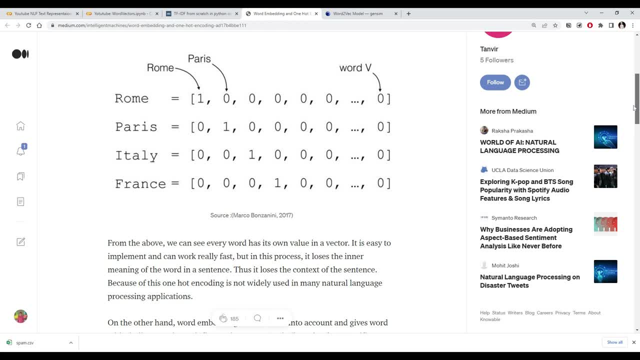 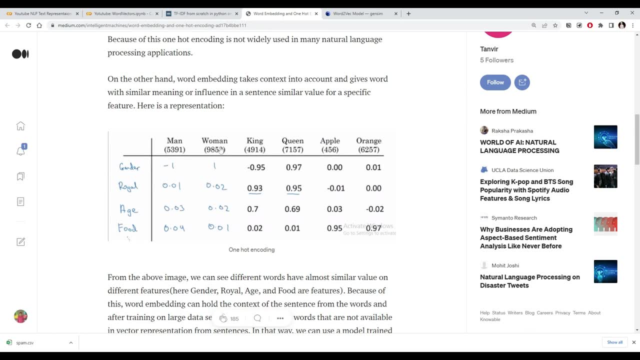 use this particular word vectors, and solve our problem. but uh, you should go and read about, you know, uh, the word to wake theory, how to train those word to wake. you know that kind of thing. you can go and read more about it. so let's go back to our notebook and what we will do. let me install. 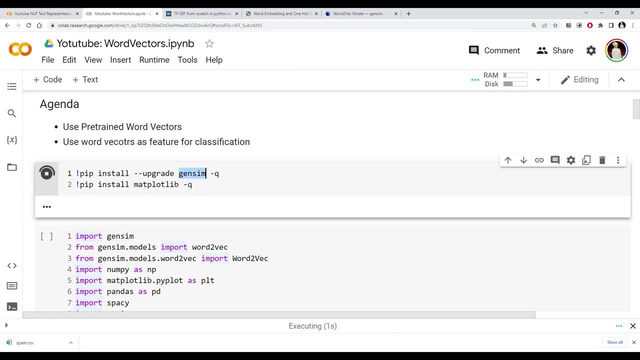 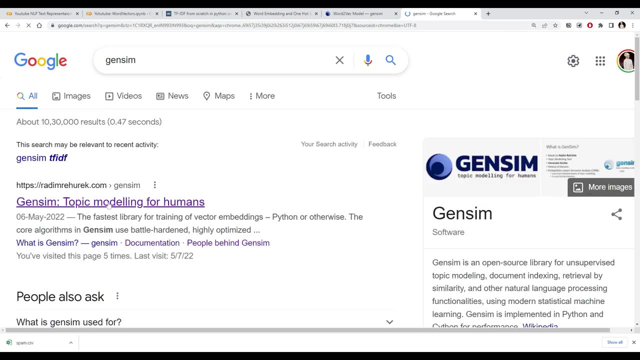 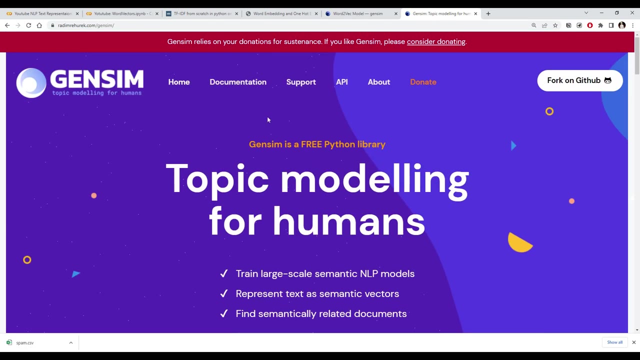 from. you know this library called chain scene. so chain sim is the library which makes us easy to use those particular word vectors, right? so gene sim has an api using which we can download some word to vectors. you can read, uh, you know documentation of gene scene, what it does. 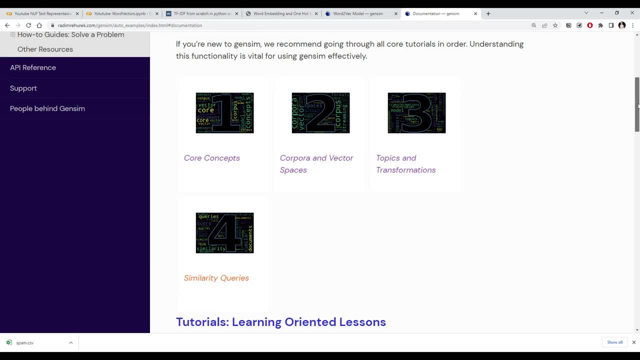 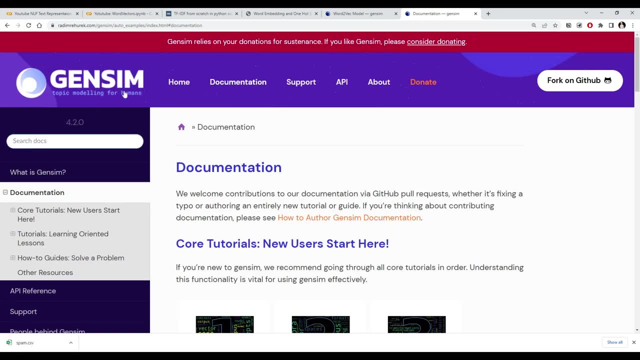 and you know what all things, especially i use gene scene for word to wake kind of thing. and the second thing, for topic modeling. gen sim is quite popular for the topic modeling kind of thing, so we will see the it's- you know what to make aspect of it. 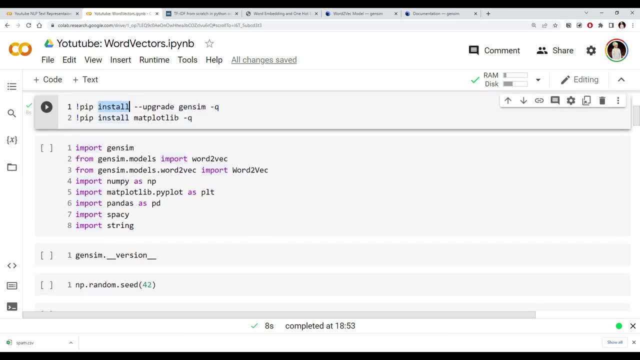 so let's, we have installed this thing using the pip, and then what i will do. i will import certain thing that i i need, so you might see there i am importing, you know, gene scene, then numpy, matplotlib or some, so you know data science libraries that we might need it right. 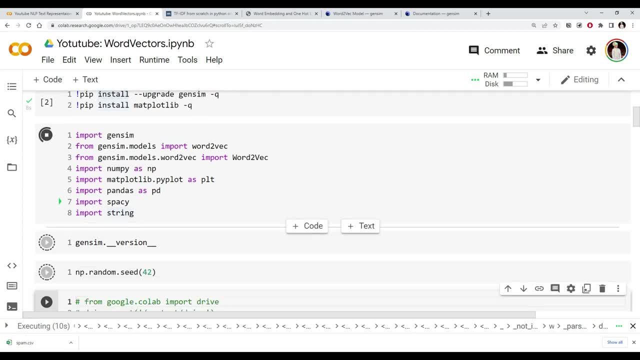 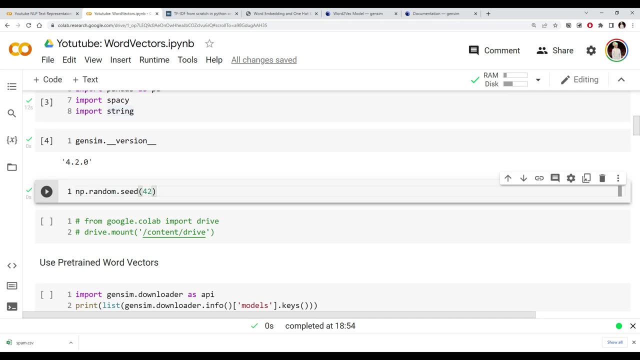 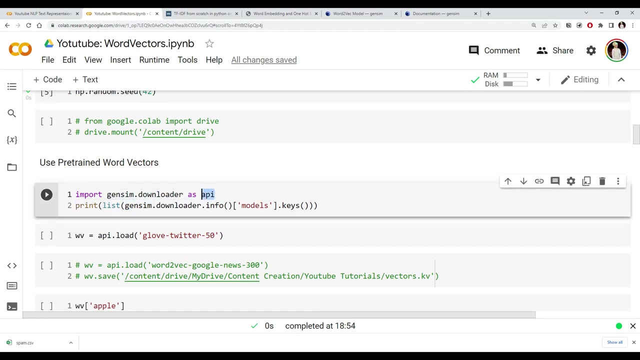 and then i'm just printing the dancing version here. okay, setting the random seed so that i can, you know, reproduce this result. now, this is what i was talking: how do we use those pre-trained code vectors? gene scene has an api. using that api, we can download the pre-trained word vectors. so someone? 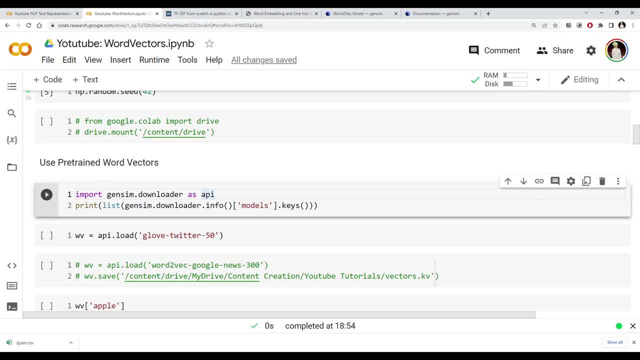 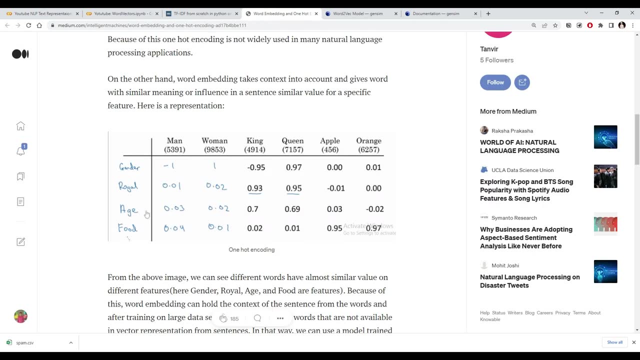 has trained those vectors on a huge data. and finally, for given any word we can get the vector representation associated with and we we can think of those vector representation has certain meaning. so that if i compare the two words and their vector representation, if those words has any meaning or, let's say, semantic similarity in real world, then i should. 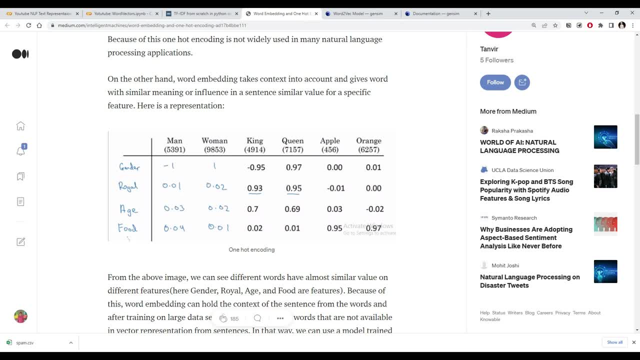 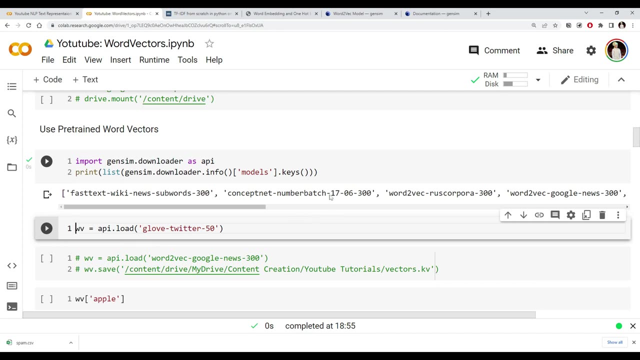 also see that similarity. if i perform a mathematical operation like a dot product on those particular vectors or check a cosine similarity of those particular vectors, you will just see what i am actually talking. so let's first of all, you know, see what are the different word to weight. models are available. so if you use the genesim downloader info. 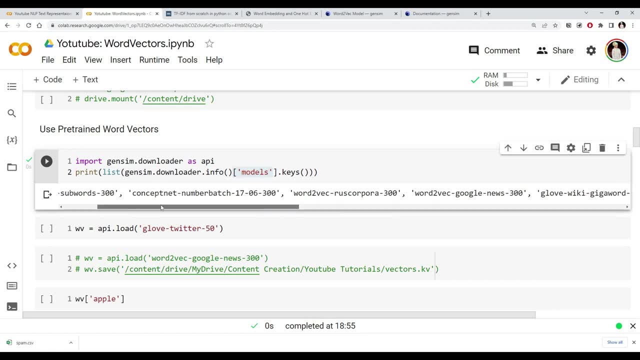 and if you look at the models, you will see what are different vectors or the vector models are available and they have certain conventions. so this is, like you know, this is one of the famous from the google, which is what to wake model train on the google news and 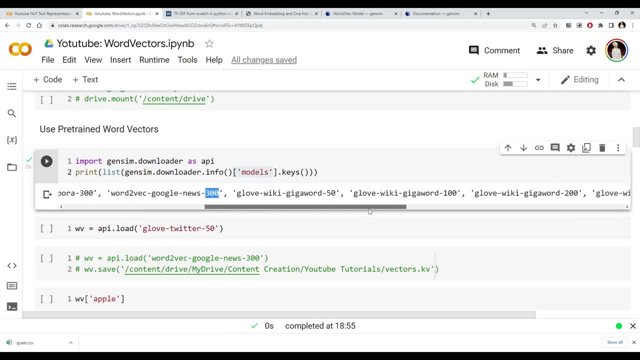 which is a 300 dimensional, and then you will have other smaller things. so this is so. the globe is also one of the technique for you know, creating the word vectors and you could see we have a couple of things. so, using this genesim downloader, we can simply use apiload and we give the name of 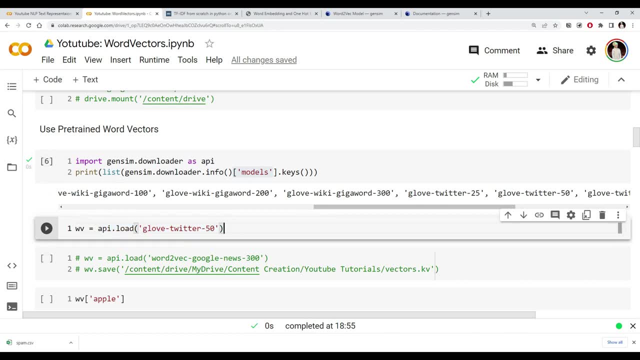 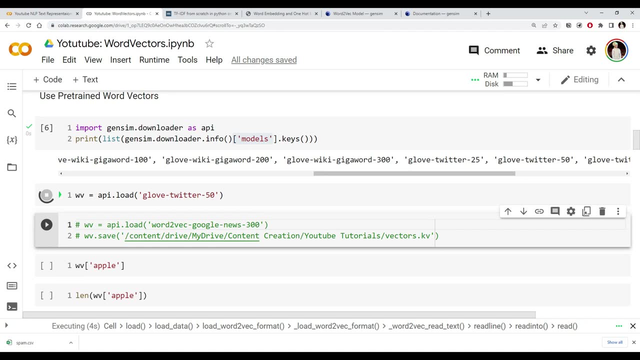 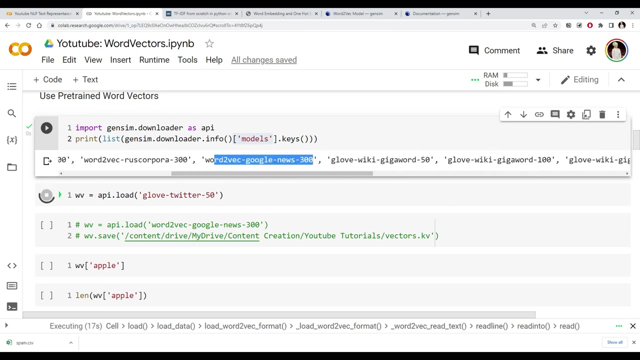 the one of the vectors that we want to load. let's load this glow twitter 50 vector. it might take, you know, a few seconds. so the thing is that this vector, if you want to load the large vector especially, let's see the google one, let's say 300 dimensional, it takes some time. 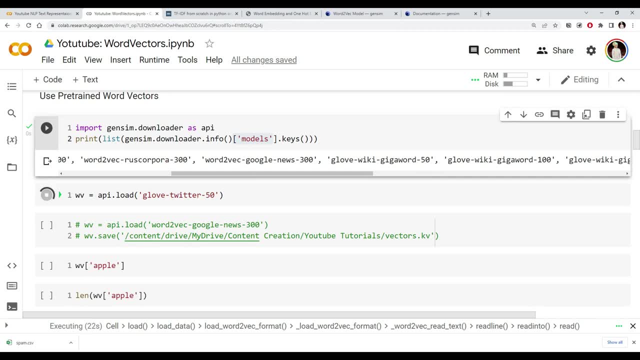 to load that particular vector. so when i tried loading it on collab it took around 13 to 15 minutes to load this particular vector and also after loading, while using, i frequently face the session crash. so i think it exceeds the ram sometimes and you know, session crash and we. 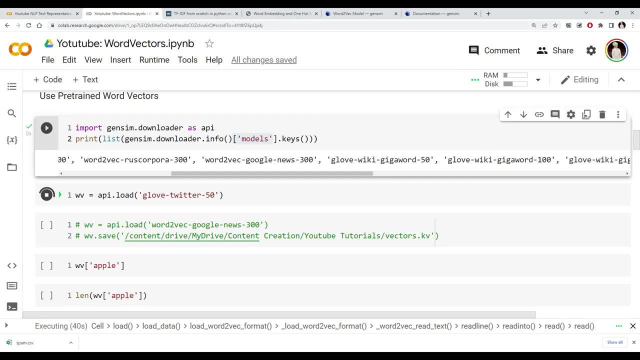 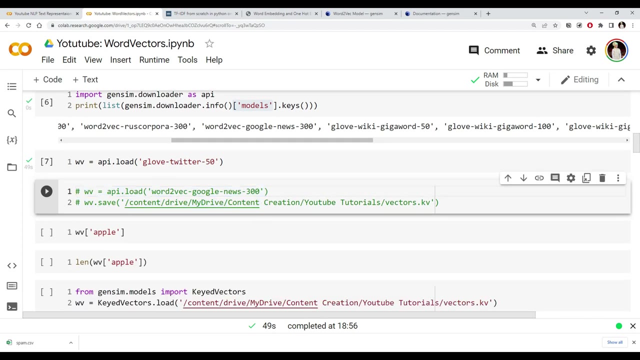 have to repeat the same steps. so what i did? actually i have loaded that particular google news vector and save that vectors here. so this is how you can save vectors. so if you load any vector like this, you can use it's a save method and give the location where you want. 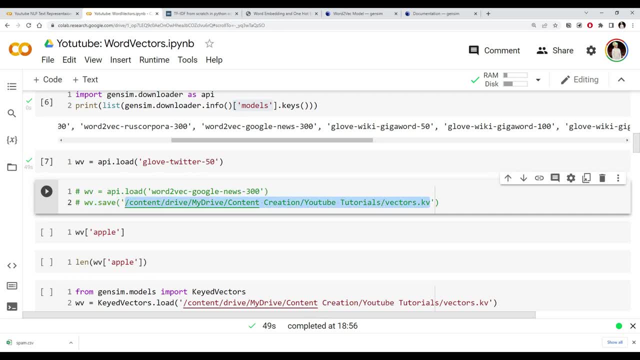 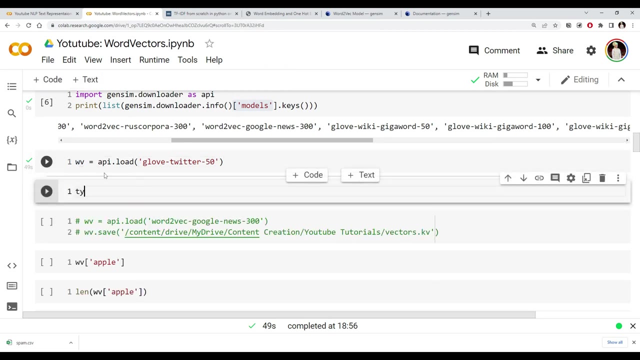 to save those particular vectors. so this is where i have saved them and we can also load. i will show you how to load them. so let's see whatever the vectors we just downloaded, which is wb, which is actually those vectors. maybe we can see what it's type. okay, you can see. 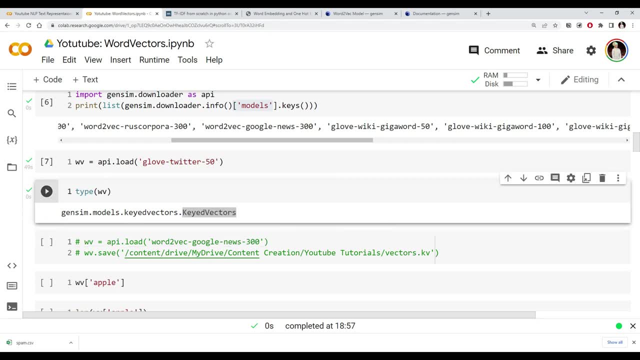 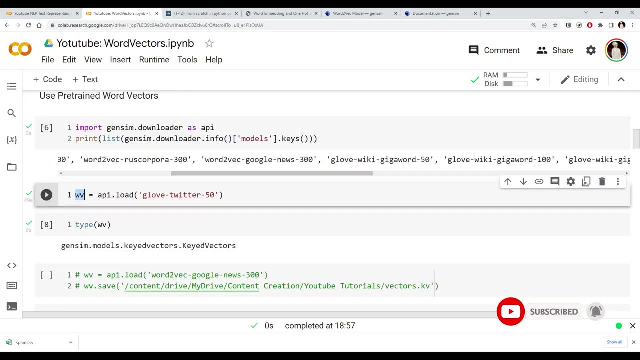 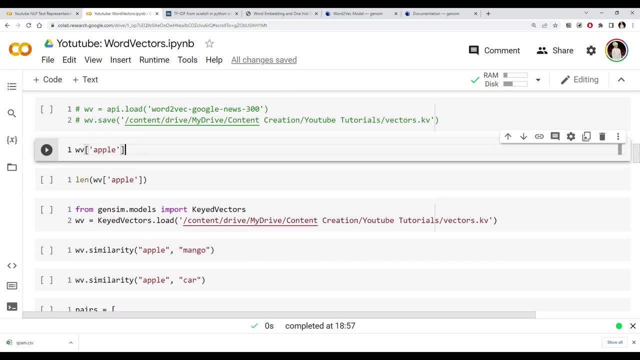 the type is something called keyed vectors. this is something the genes in type, what we have now, what we will do this vector, what we downloaded it like a lookup or a dictionary you can think of, you can pass any word to it and it will retain a vector representation of that word. that's. 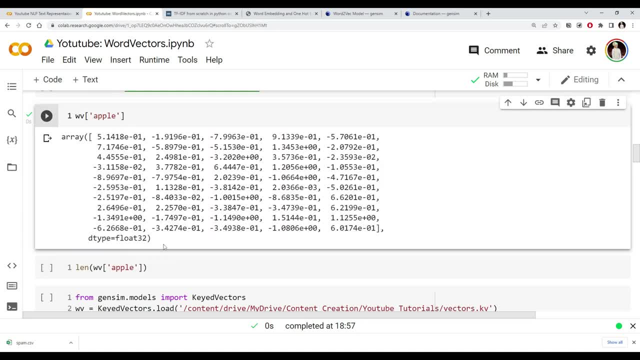 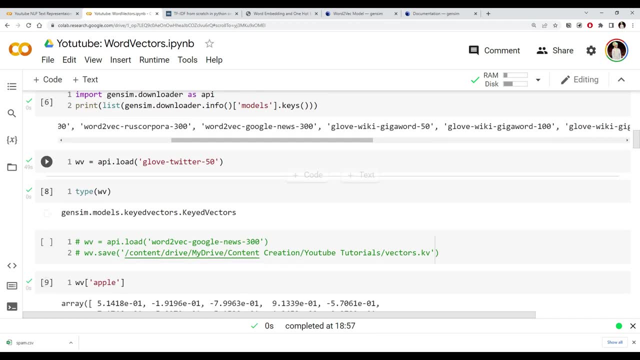 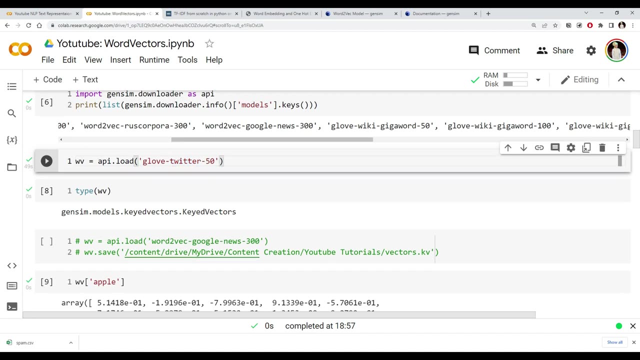 it's something like a lookup so you could see we got some vector representation. look at, look at the length of that vector. we see the 50. why? because we have downloaded that a 50 dimensional globe vectors, which was trained on the twitter data. but when it comes to, let's say, 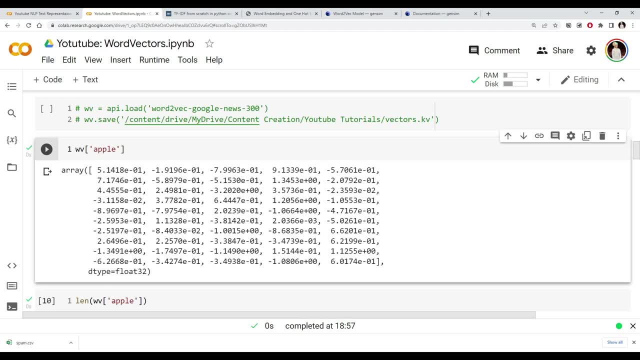 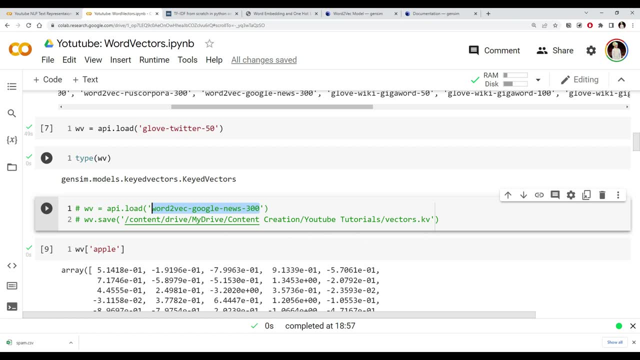 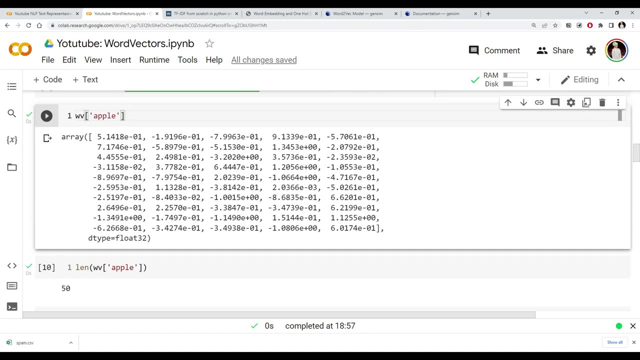 the accuracy of those particular vectors. it's always better to go with the- uh, you know what i could say- go with the bigger vector representation, like this particular vector representation. so let's see what we will do. we will try to do some operation using this vector right, and i will not load that thing yet. so this: 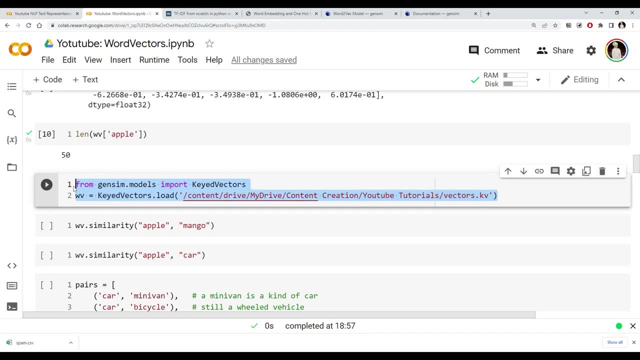 is where i have loaded those 300 dimensional. let's forget this for now and let's compare what we just did. so we we can ask our word vector to tell the similarity between these two particular words. so it has a method called similarity. so let's see what is the similarity between, so we can. 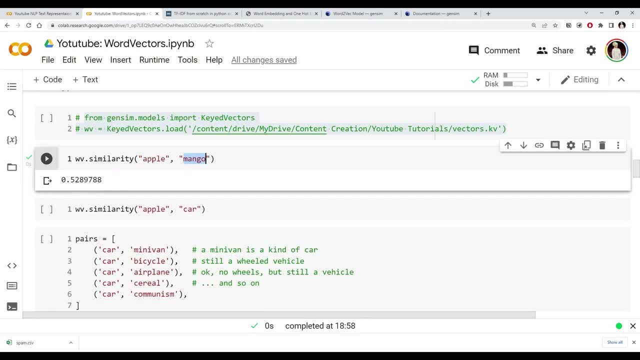 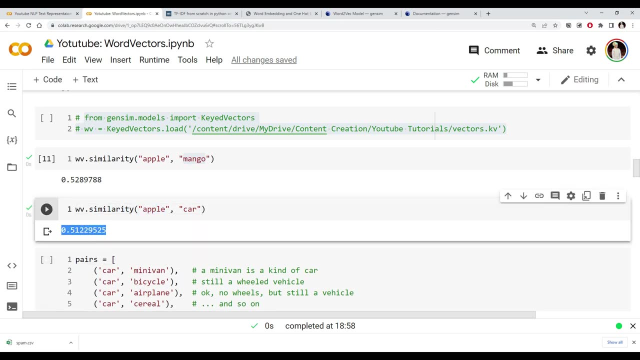 see the similarity between apple and mango, which is 0.50, and let's see the similarity between the apple and car, which is 51. doesn't seems to be good because we know that apple and mango are much more closer to each other compared to what apple and car, so we expect we should have a high. 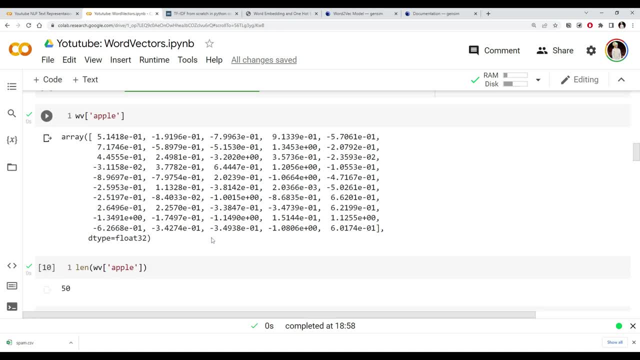 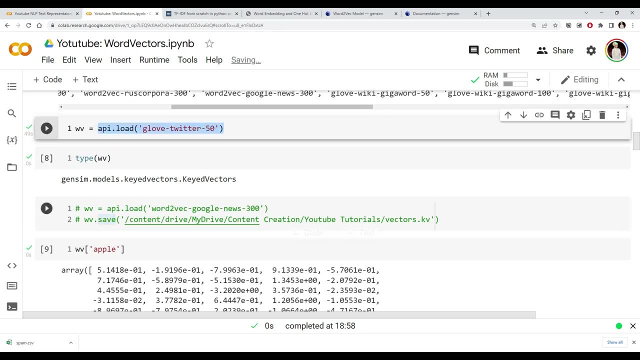 similarity here and low here. maybe we can try using our bigger vector representation right, which i saved the similar way. i simply load them and then save them here and once you save you can use the load meter to load them. so let me load that particular vector so that we get the bigger. 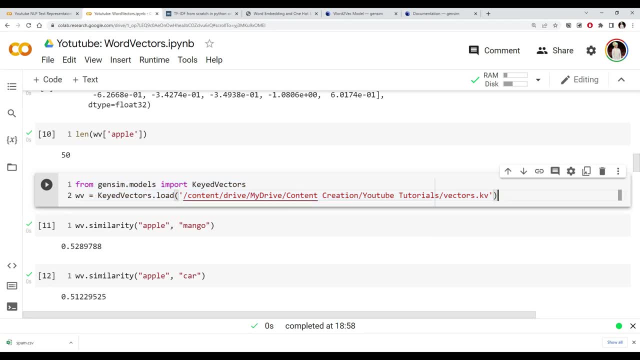 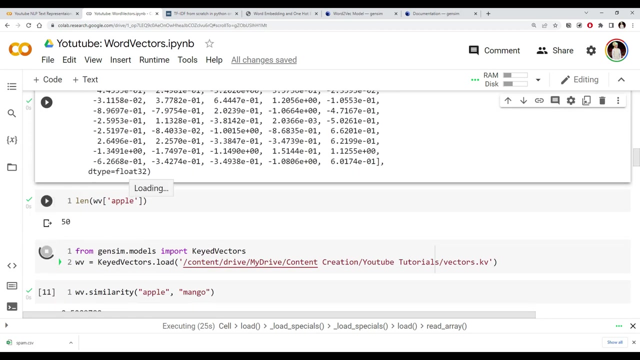 vectors here and again. as i said, it might crash a session and then i have to repeat these steps again. so it's loading. once it load, we will execute these two cells again and and we will see the dimension of that particular vectors, what we are loading. so 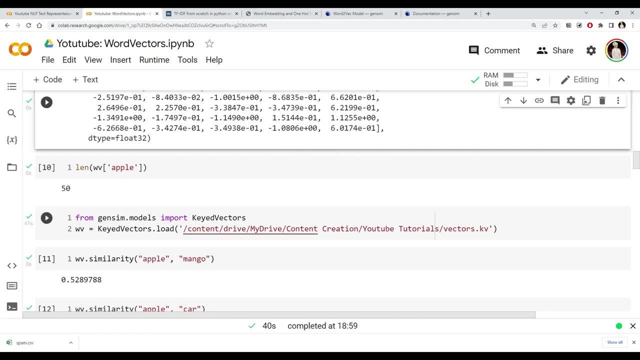 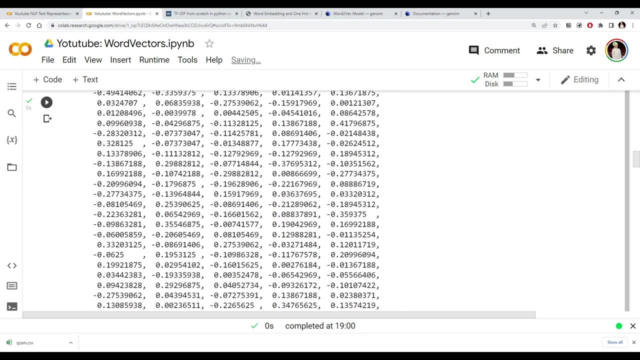 okay, it has load. i think it loading took 40 seconds, but if i want to download this thing this might take a 15 minutes also. so let's see now again, because we have stored in the same variable wb. now we see we have bigger vector representation. let's look at the length, which is the 300. 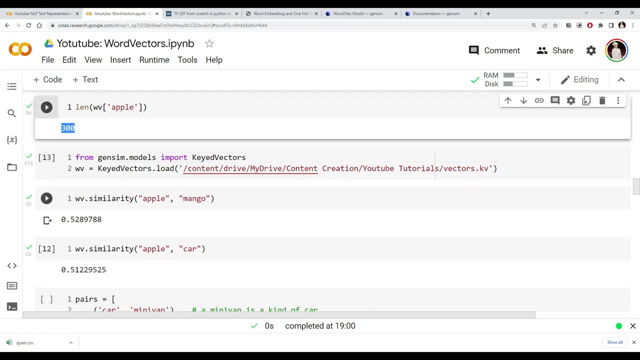 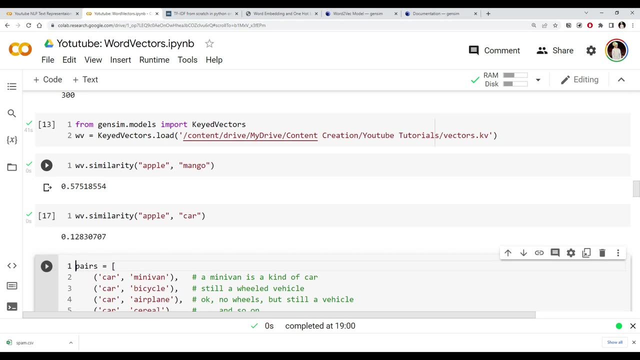 dimensional. that is what the google vectors, what i downloaded. now let's check using those vectors, what's the similarity score for apple and mango and what is for the apple and car? now you see, it is much more meaningful. so definitely the bigger vectors, larger vector, 200, 300 dimensionals are way better than those 50 dimensional vectors. right, because now this: 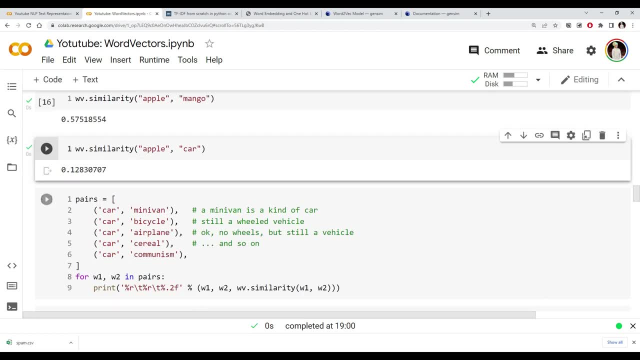 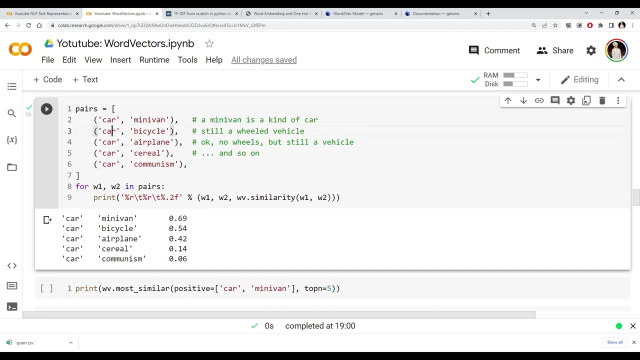 is something, uh, what we were expecting. just like we can check a similarity, let's check a similarity here pairwise. so we have a couple of words- car, minivan, and, and some of them, and you could see we got the highest similarity between the car and minivan and then you have very 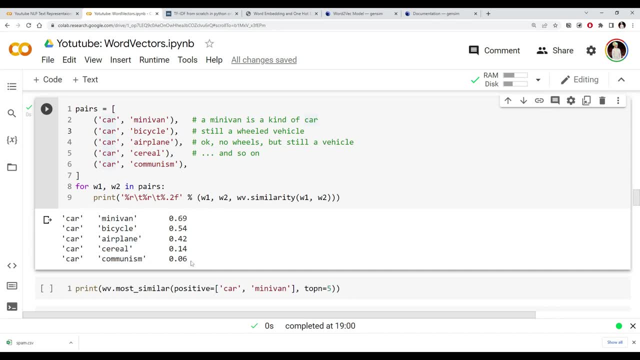 less similarity for the other word, the car, and communism and all this thing. so definitely. this is what i mentioned at the start of the video- that if there are two words which has some semantic similarity or or they have a similar meaning in the real world, we should expect the 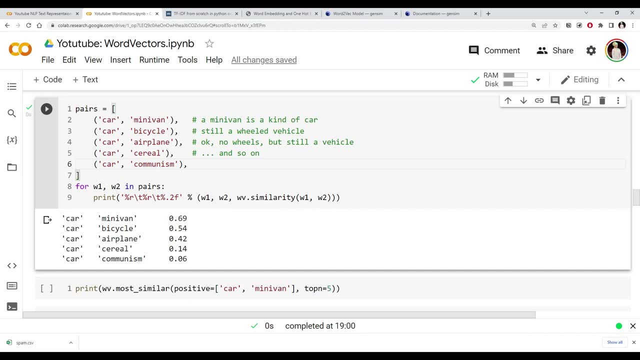 same similarity when you compare their vector representation, and that is what we are currently see. we know that the car and minivan are much more closer in the meaning in the real world compared to the current communism, and that's what it is reflecting here. another thing is that 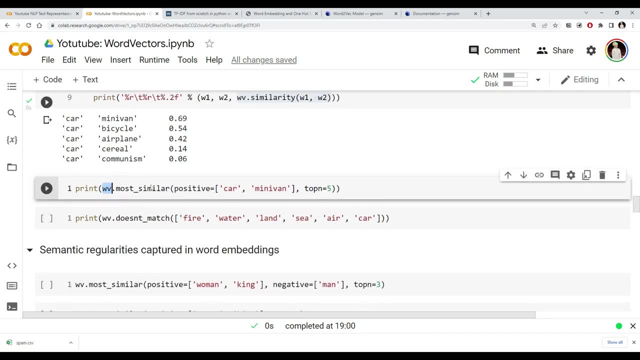 using word vector we can also check, just like similarity, we can also check what are the most similar words for given my words and you can tell that whether you want these words. so there are two ways you can specify those words. you want them, the new words to be the. 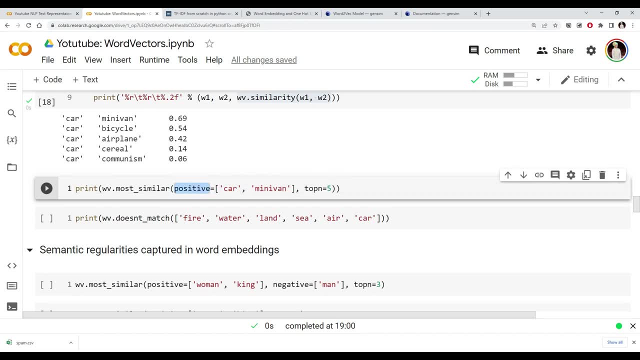 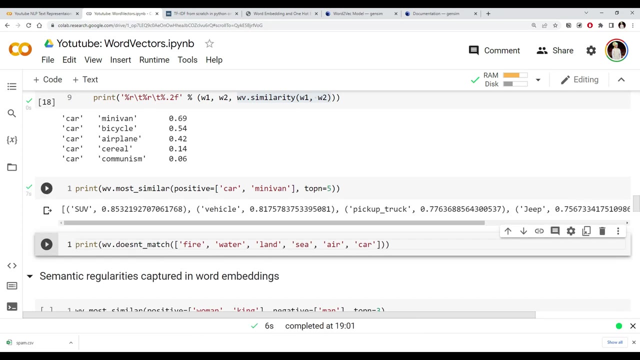 positive towards this particular words or the negative towards these words. right, so positive means the new words. we want to be similar, like this particular. let's see what words we get. similar to this: car and minivan. okay, we got a word called suv. we got a word called vehicle pickup truck, and you could see. 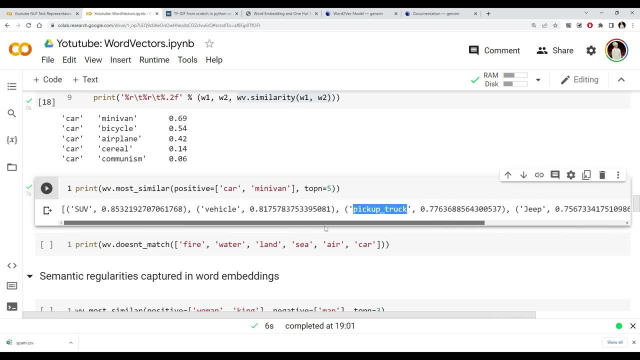 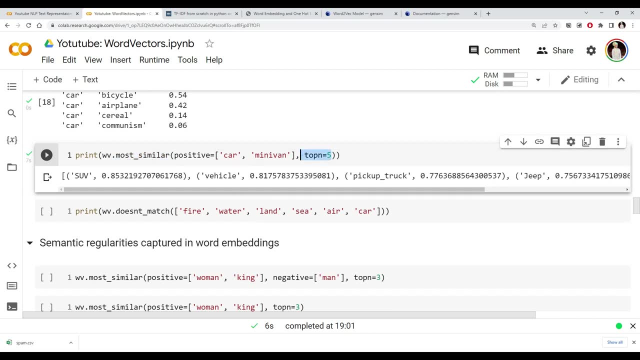 all of them are some vehicles, right? so this is how you can generate the similar words given any particular word, and we specify that i want to see the top five words. each word we got similar to the above words and also we got the score associated with it. you can also think you know that among 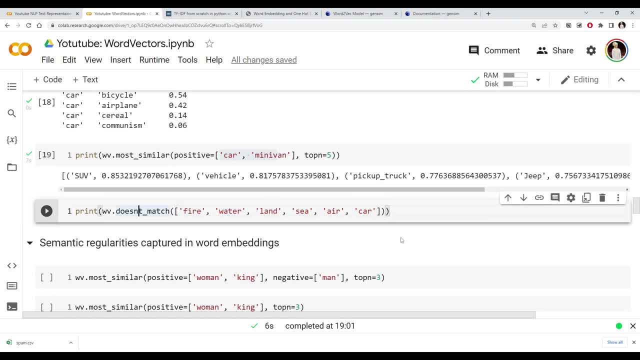 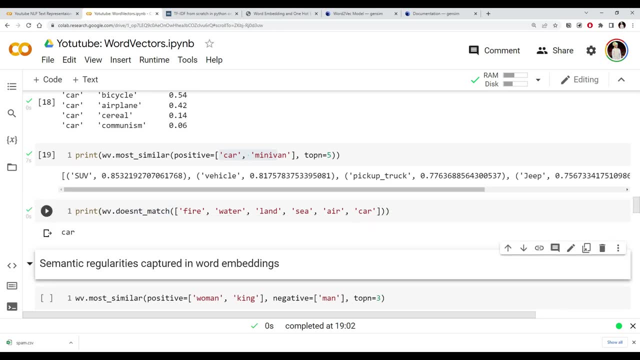 these words: which doesn't match with the others. so i think it's odd out or odd one out, kind of thing. right, that is also you can check. so these are all. uh, you could see out of all this word. it's saying that the car doesn't match with the other. 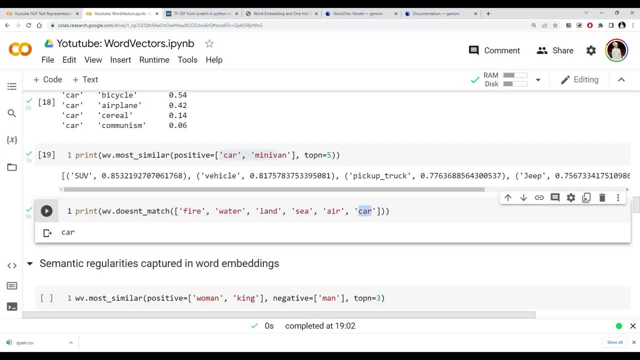 word, because all are natural elements and this is something car you can think of, it's a man-made or the man-made, uh, particular, you know, uh, whatever that object. so this is see how powerful and beautiful these vectors. you can check the similarity, you can find out the, you know, similar. 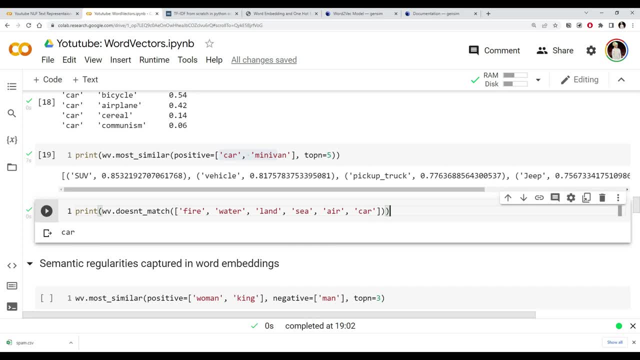 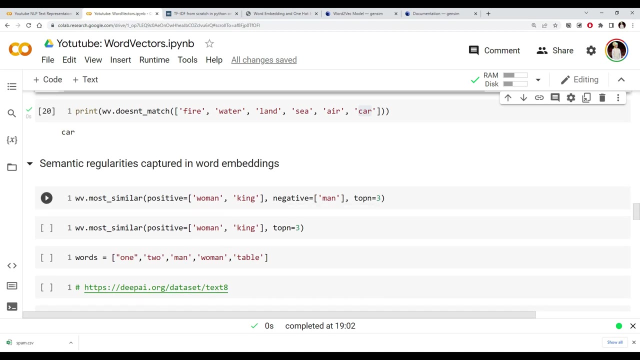 particular word and you can even check whether you know particular word matches with the other word or it is odd among the others. let's look at this particular aspect again. you know that positive thing. so let's say we want to find a similar words which are positive towards the. 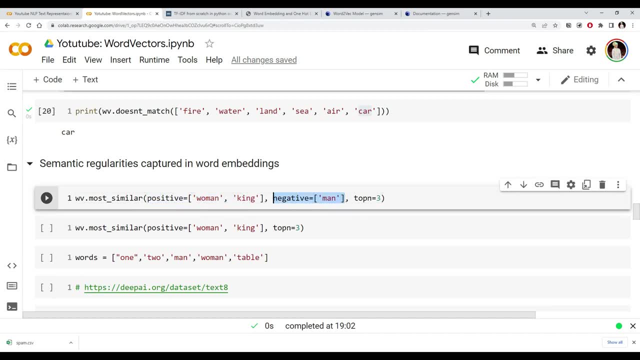 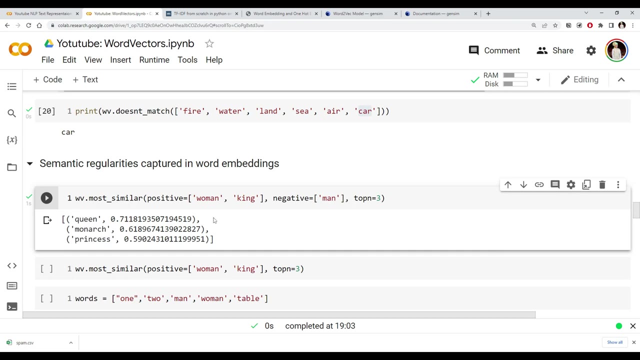 woman and king, but they are negative towards the man. so we want those words should have similarity, these words, but they should be away from this word. so let's see what happens. so we got queen, monarch, princess. these are the words that it is related to the women and king, but away from the. 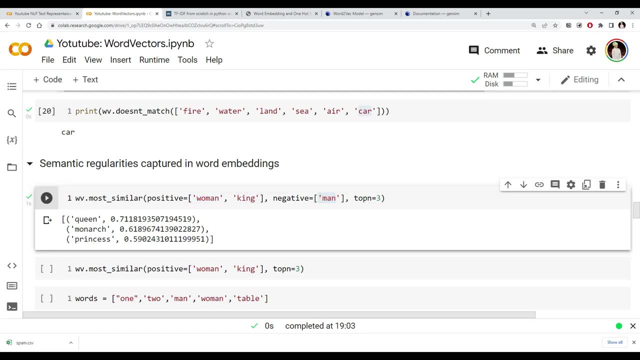 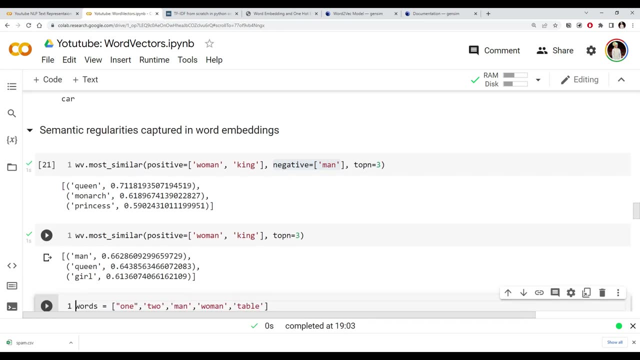 man. so you might say that these are all related to the female gender. right? what will happen if, if you don't put this negative aspect here, what things we will get. you see, if i don't put this thing, then i get the similar words for women and. 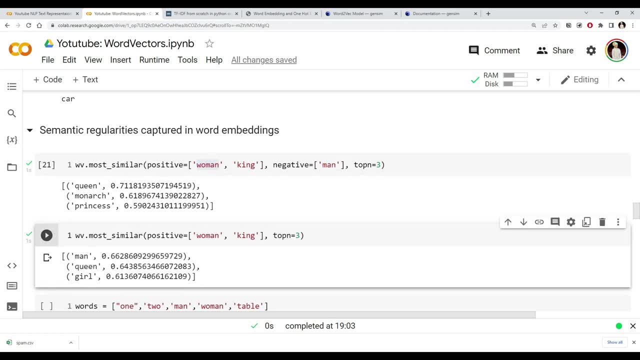 king like a man, queen, girl. so we see man is appearing because it is definitely similar to the king or has some contextual similarity with the women. but when you put something negative- so we want something which is close to women, which also has a king aspect- you can think of it so. 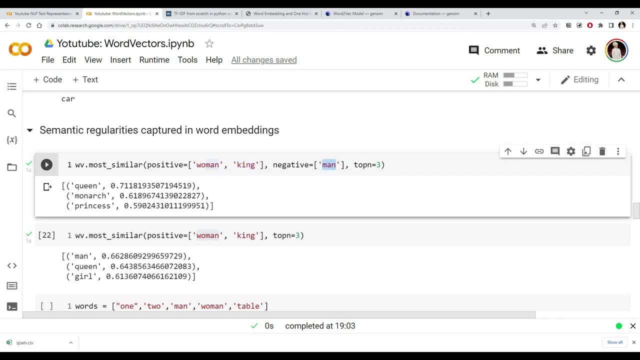 you want king aspect, but you don't want man. so what is remaining? if you subtract man from the king, the things remain only the royalness. so you have a woman and the royal. that is why you see the queen and princess appearing here. so this is how beautiful. it is right, and these are the famous. 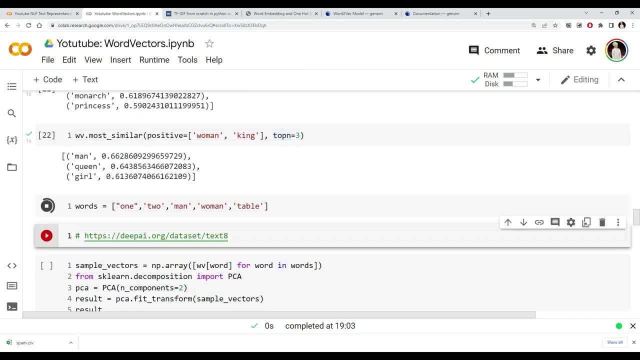 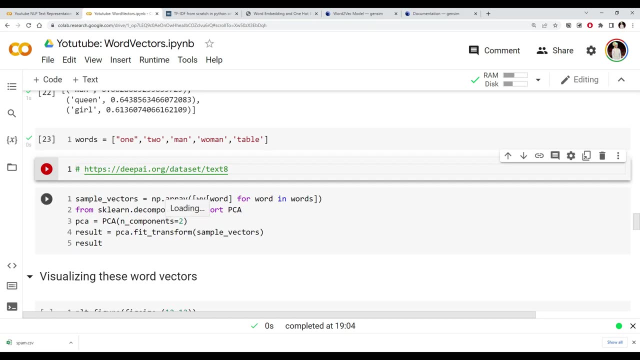 examples. another thing is that let's take a few random words. i pick up like one, two man, woman and table and what i will do. we will try to visualize them right. but since we can't visualize those 300 dimensional vectors, then what we will do, we will use pca, which is in a principal component analysis. 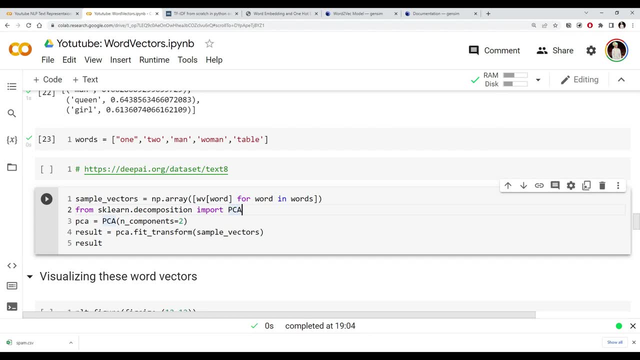 which is nothing but dimensional reduction, dimensionality reduction technique. so we want to reduce the 300 dimensional to only two dimensional, so that we can see here: it's fine, if you don't have used this particular thing, just ignore this thing. just see whether what we see here right. so what we did, every word. 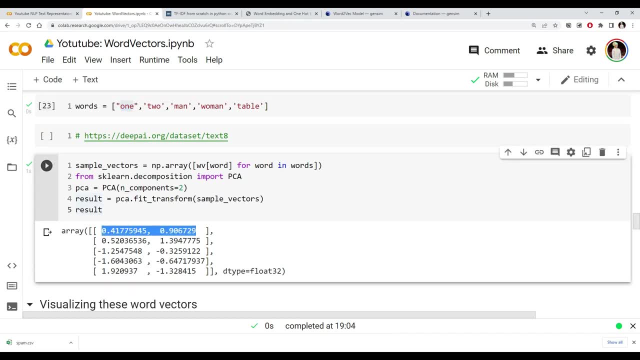 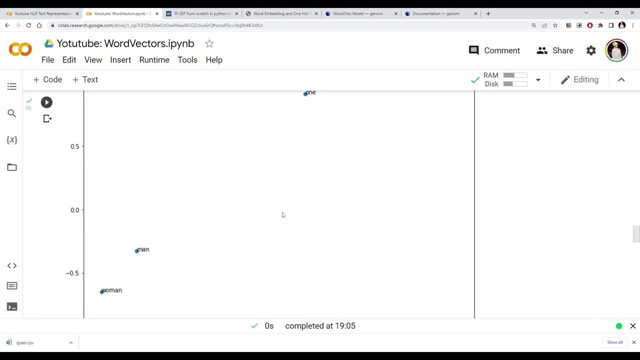 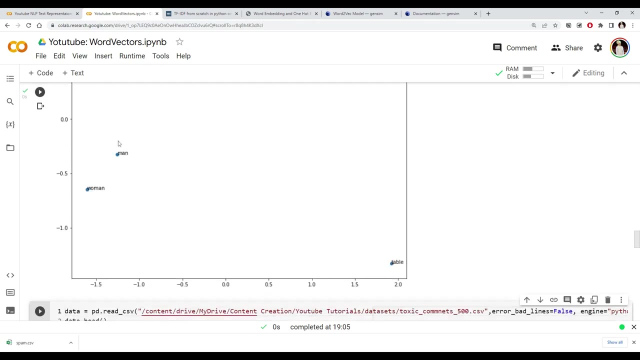 instead of 300 dimensional, we reduce it to only two dimensional and then we will plot those words and we will see whether we could see something interesting there. you can see when we plot these words, let me you know. okay, you see, in this particular plane woman and man come somewhat closer compared to where the table. 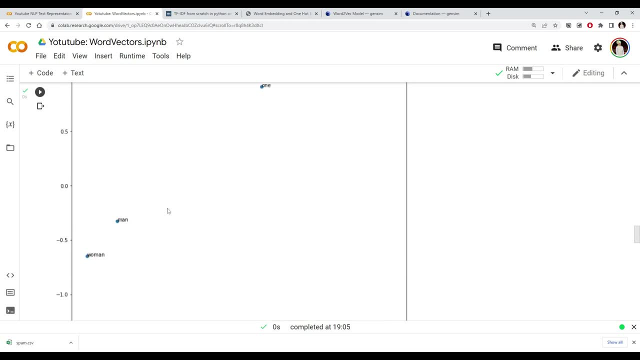 which is far away from so definitely. even on the two dimensional, we can see that vector representation still has some semantic meaning with respect to a real world that we see. women and men are closer in the representation and you know, one and two got closer because they are numbers, these are genders and this is something totally different from them, right? 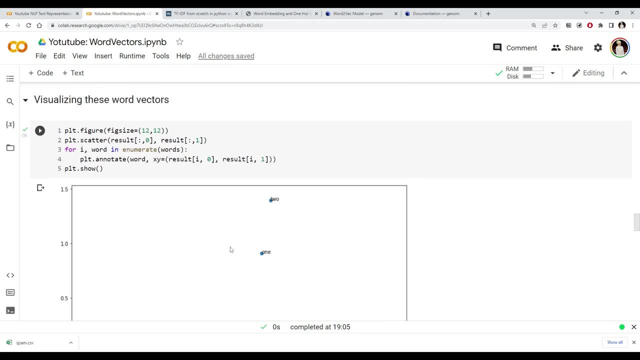 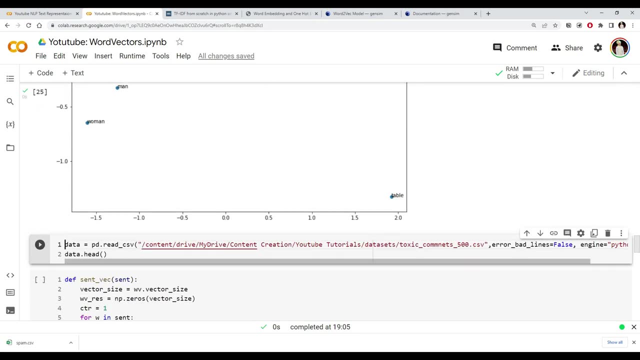 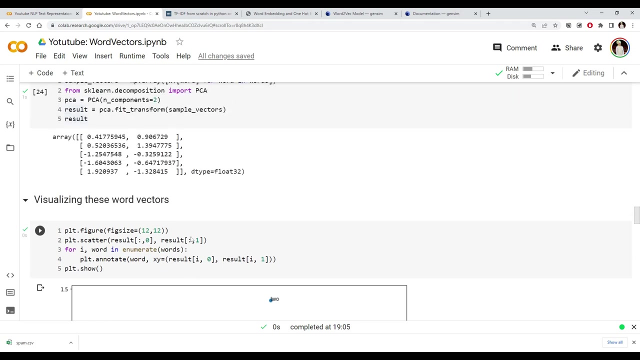 so this is what you see, even when you reduce them from 300 dimensional to the 200 dimension, right, sorry, not a 200, just a two-dimensional. right now, what we will do? enough. now we have a good vector representation for a particular word, then let's try to, you know, build a classification model. what? 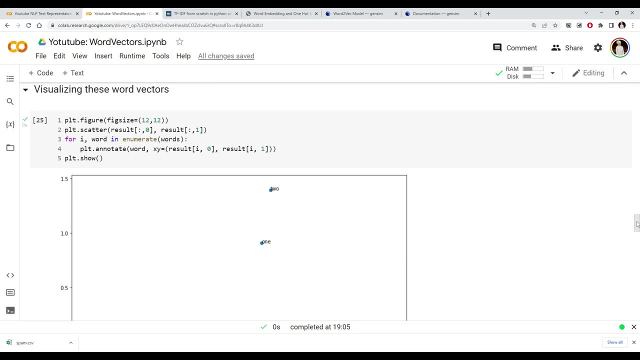 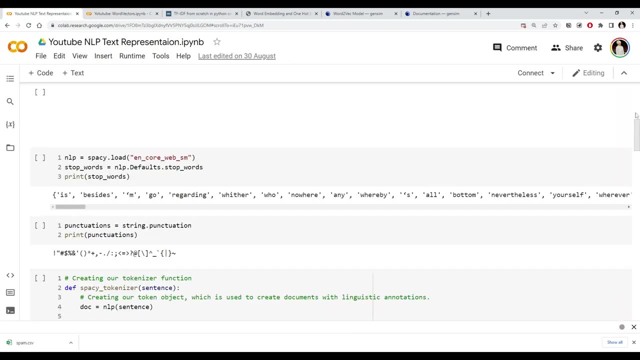 it will do. it will represent our text using this particular vector representation. so let me first load our data, which is the same thing, what we have used in our previous video, which is that toxic comment. you know, data set where you have a comment and we tell whether that comment is toxic or not. 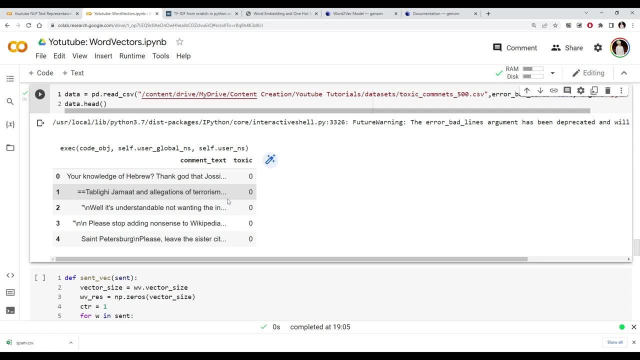 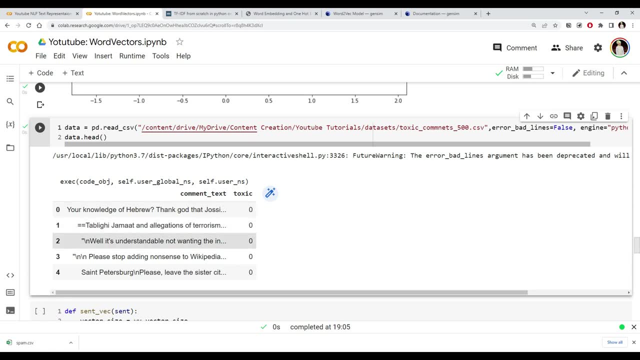 we have. but the thing is that we just saw that you have a representation for a word. so if i you pass this particular word, let's say this, you will get some vector associated with. if you pass this, you will get some vector. but how do we represent the sentence, right? so the one way is: you can take. 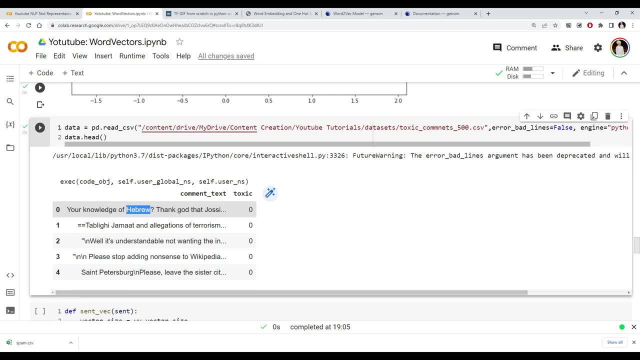 vector representation of this, concatenate with the vector representation of this, and you can do this thing. but the problem with this thing is that then your representation for a single sentence will depend on the number of words you have here. so imagine you have a 300 dimensional vector and 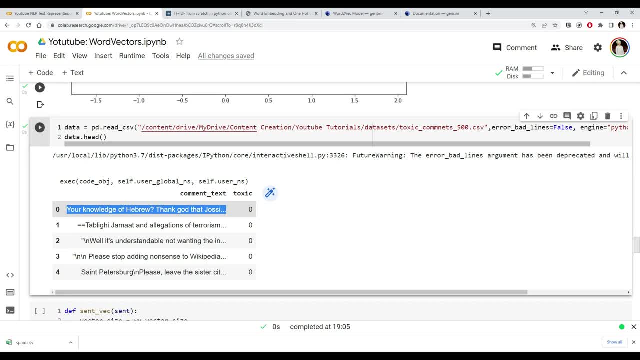 there are 10 words here, then it will become 3000 dimensional vector. but what if here you have 20 words? then it will become 6000 dimensional vector here. so this is not going to work. you need the sentence to be represented in all the sentence to have the same length when you represent for. 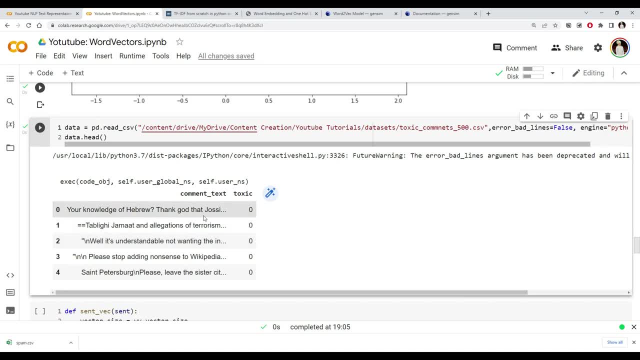 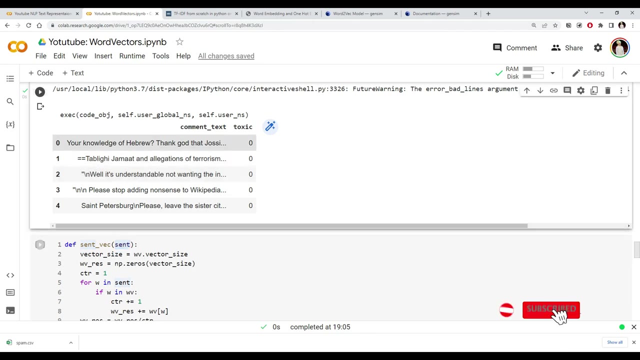 the machine learning. so that is the reason that might not be a good approach to concatenate what other approach we have. we might do a summation or you can take an average of the word. so what we will do, we will go with the average approach. we will take our each sentence. what we will do, we will find each word in that sentence, get its. 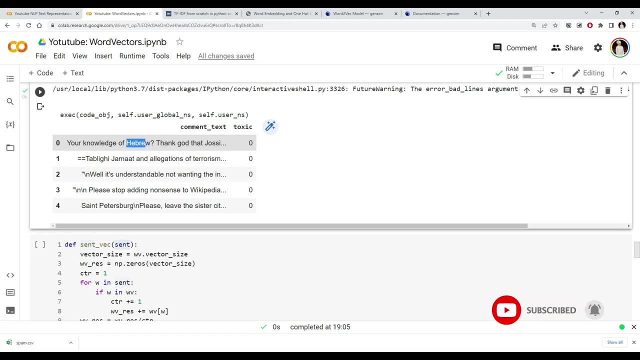 vector representation and keep adding all the words and finally take the average of those then. so the final sentence representation will be having the same length for what we had for a word length. so ultimately we should get a sentence with the 300 dimensional and each sentence will have. 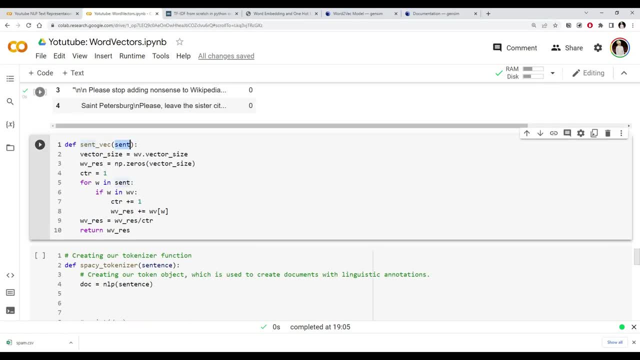 the same length, the 300 dimensional vector, right? so this is what we are going to do. we are going to do is take a sentence and we have our word vector. we see what is it? vector size. so it has one of the attributes called vector size, so this will be having value 300. then we need to use numpy and 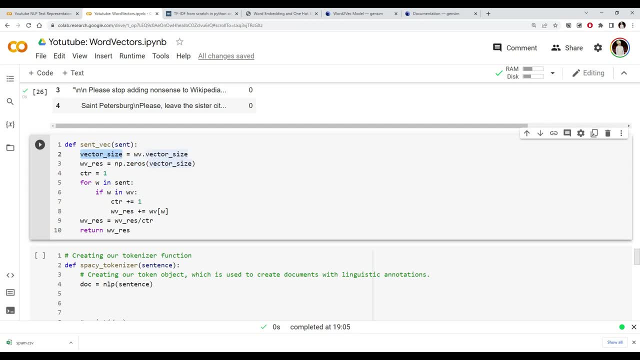 create a big vector of a length, this vector size. so here you get a vector size of 300 dimensional. all will be the zeros. then what we will do, we will iterate through our sentence. this is what we will do for w in our sentence. or let's say: whatever the tokens we have, we will see the, do we? 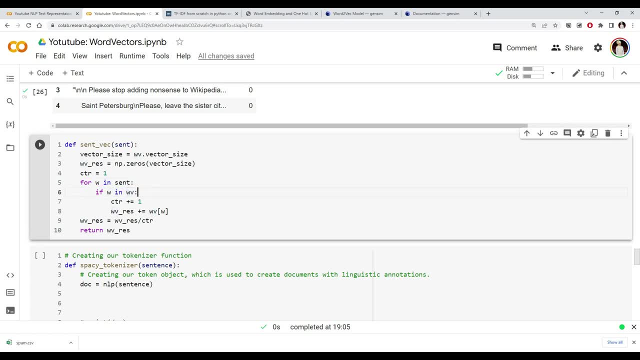 have that particular word present in our word to wake. if it is there, we count, increase the count because we want to take average this way. that is why we want to know how many words were in that sentence. and then what we will do. our zero vector: we will add the vector representation of this. 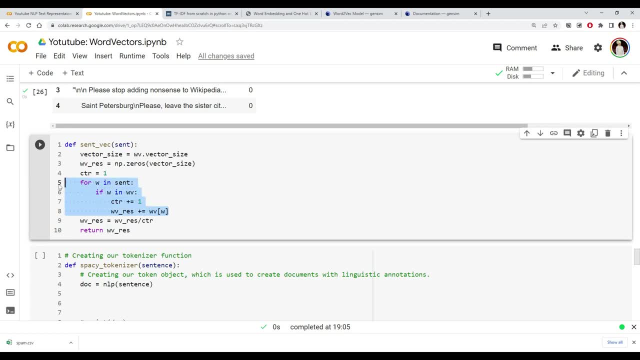 particular word. so when you complete this loop, you have eventually add all the vectors associated with each word in that sentence in this final vector and finally, you divide by the number of words and this way you are able to get the vector representation, which is equal to the summation, or, sorry, the 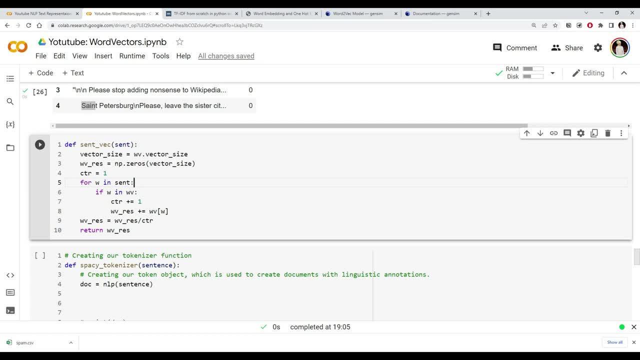 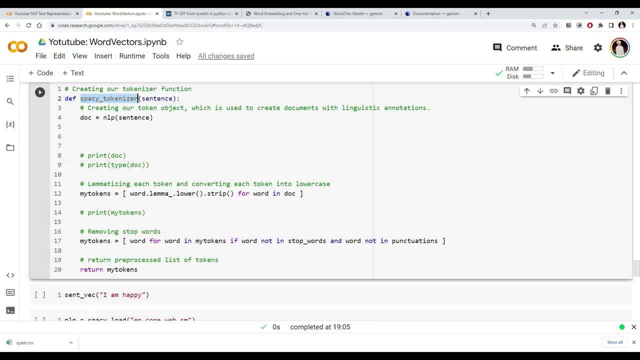 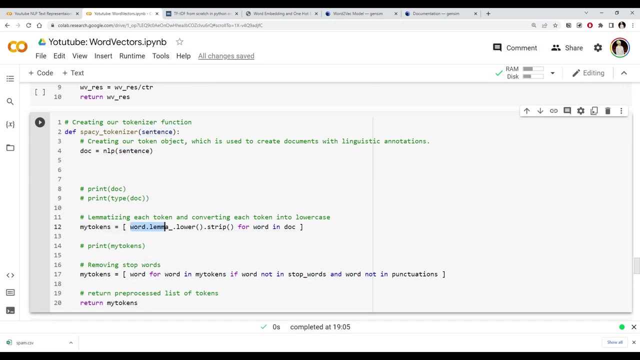 average of all the word vectors inside that particular sentence. also, this function- you might have seen the last time- which is the we have used for the specie tokenizer. what does it does? what does it do? it simply take a sentence right and find the lemma, which is the root word for all. 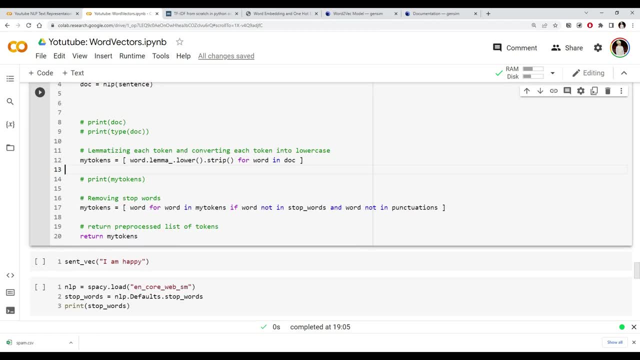 the words and then does some basic check it: does this word is a stop words? is it equal to the punctuation? if it is, we don't want to take it and we only take the words which doesn't match to one of them. so this is how we are filtering our stop words and 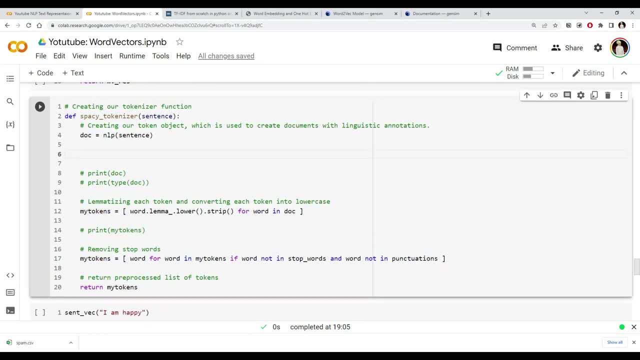 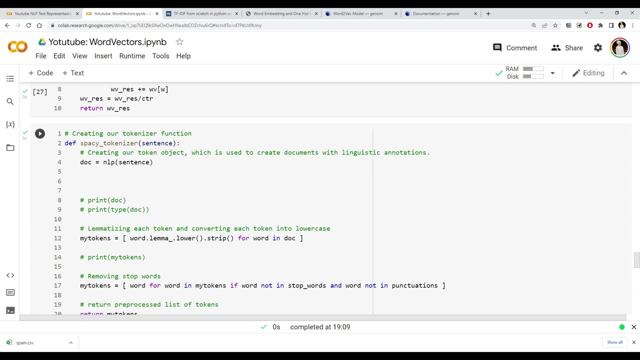 punctuation art. so that is what we have seen in the last time also. so we're going to use this. both of this function, right, so let me execute this thing and let's see what happened. this particular, this sentence vector- right, so we can pass any sentence to it and we will get the vector. 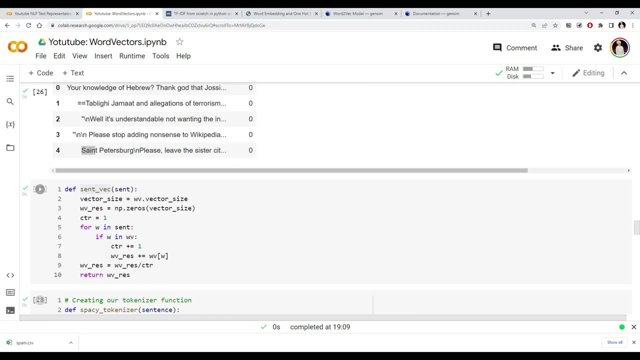 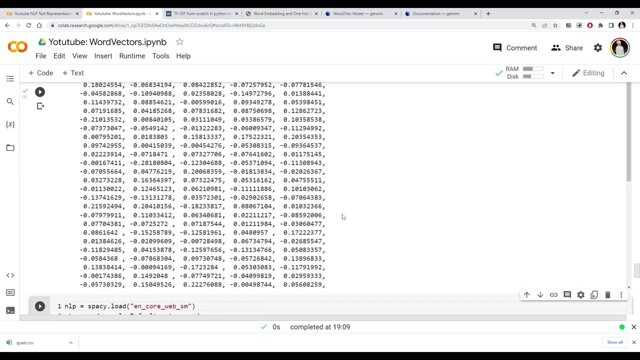 representation. should we print any intermediate steps here? maybe you want to know what is this? what we got right. so let's print this thing, this should be a zero vector, that particular thing, let's run. okay, you see, initially we declare everything as a zero and then, finally, we modified which? 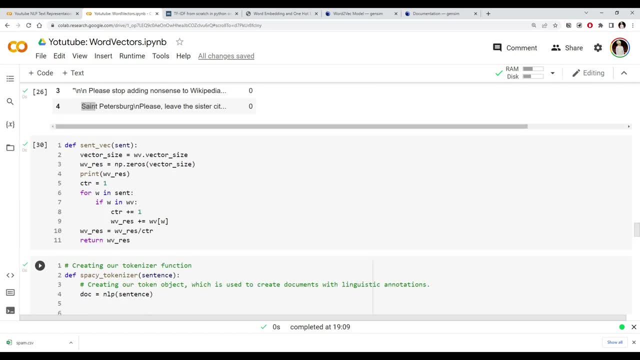 is nothing but the average of all the word vectors inside that particular sentence. so let me comment it again. so now we have a capability to take the sentence, thank you. now sentence could be this sentence also, or it will be a list of tokens also, because in both the way you can iterate, even, it is list of tokens, you can iterate and even. 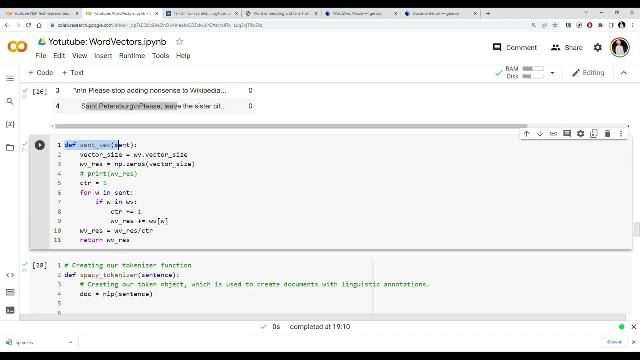 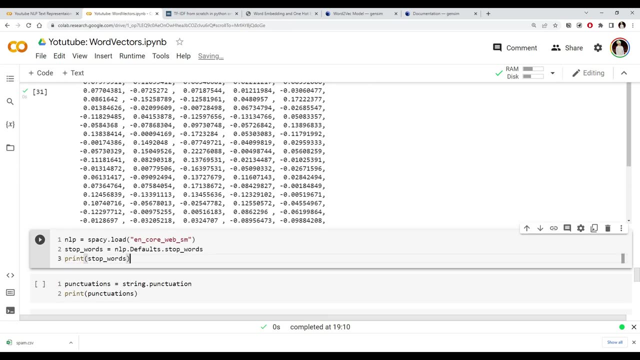 you know. so we want to pass actually the list of tokens, which is nothing but the list of words that we will get. so let's do that thing. what we will do: first we want to stop word list because we are using them on the top right, and then these are some of our punctuations. 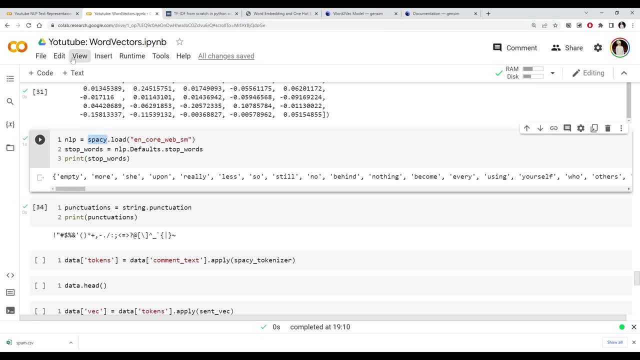 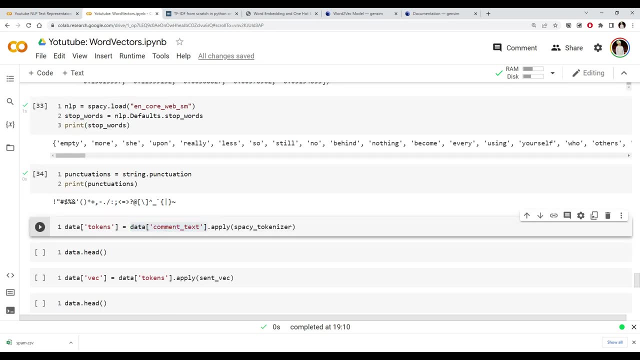 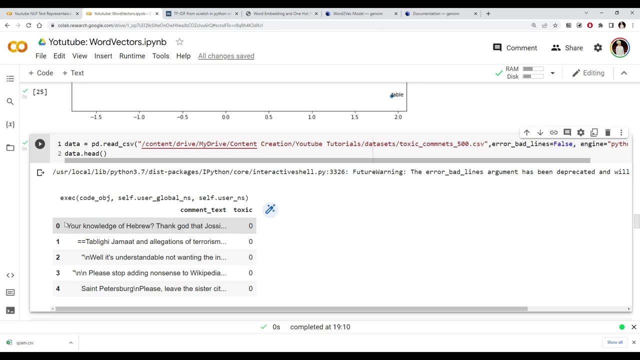 which we are taking from this spacing. we have seen this thing in our previous video. nothing big deal. now let's do one thing. we have our comment text in our data frame here. let's first tokenize these things. so, instead of having this big string, we should get the list of words and we we will be filtering the stop words and all punctuation, all. 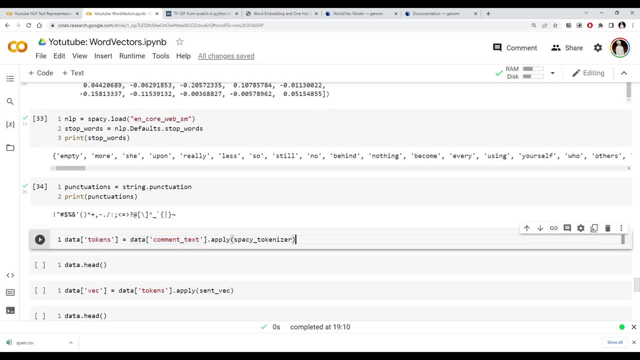 right. so let's run that step. it might take some. so you in a pandas, you can do something like this: you take that column and you apply the function that we want to apply and it will return return value in a new column. i call it as a tokens. so let's run this thing so that things will be much more clear what we want to achieve. 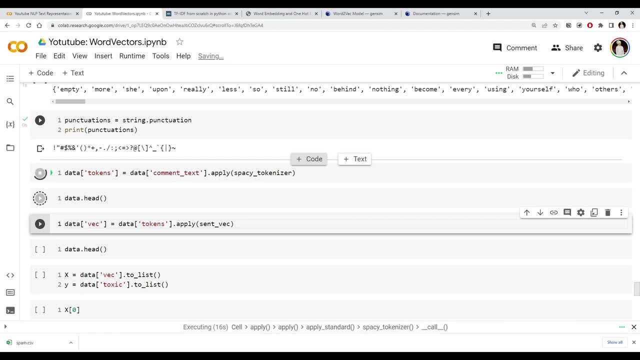 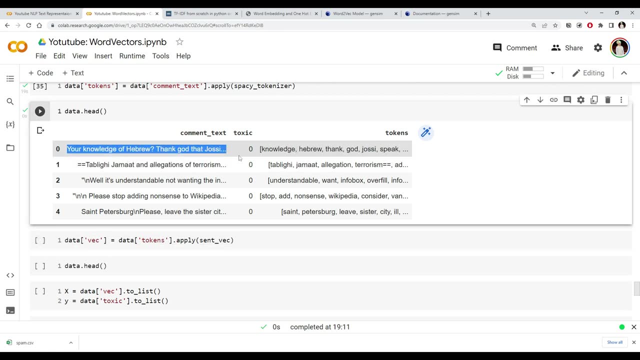 it might take few seconds to you know. convert our text into the tokens. now we will see. this is what i am saying. so it took our sentence, this, take comment and then convert it into the list of tokens according to our that function, and it has removed all the stop words that we don't want. 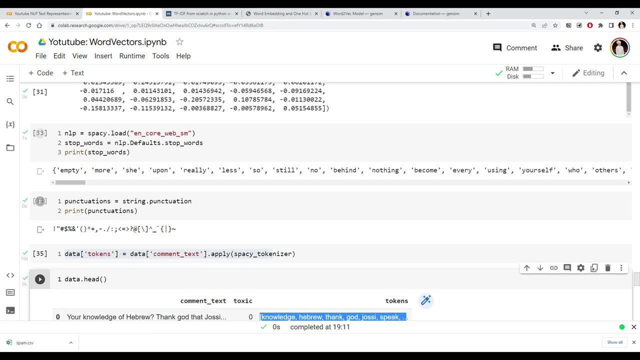 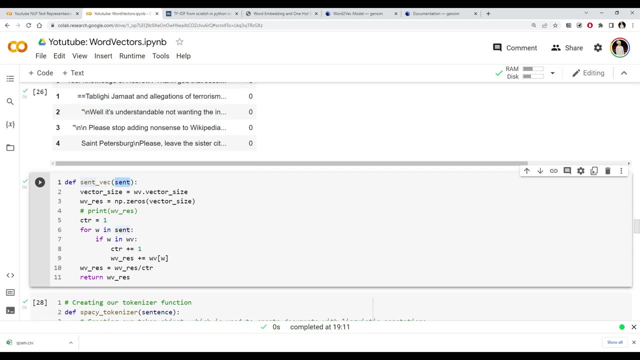 once you have our tokens, then we want to pass our vector thing, which is here, this one, sorry, this one, which take our sentence, which is nothing but list of tokens. that is why we are able to iterate through these words, because we know that is the list of words. 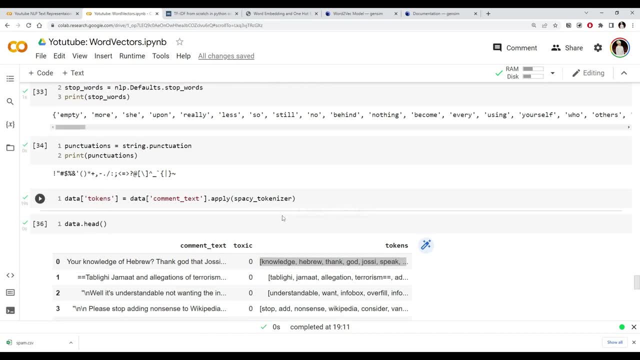 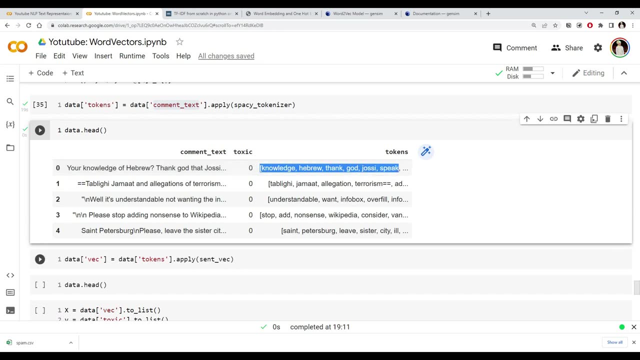 what we are passing, so this, you know. let's pass similar way, just what we did with the comment text. now we will perform function on this tokens. so let's take these tokens and apply the sentence to vector so that we can get the average vectors of this thing, and let's do that thing. this also might take few seconds. okay, it finished faster. 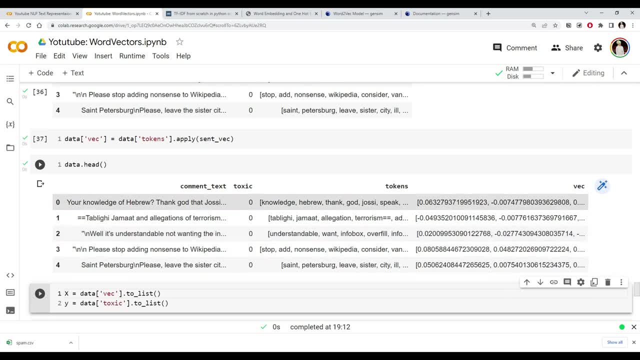 and you see, now we have a vector column which represent a vector of what we have here, right? so this is nothing but our training data. now we have each our comment represented in a vector form that we can pass to our machine learning algorithm, and what we will do. i took 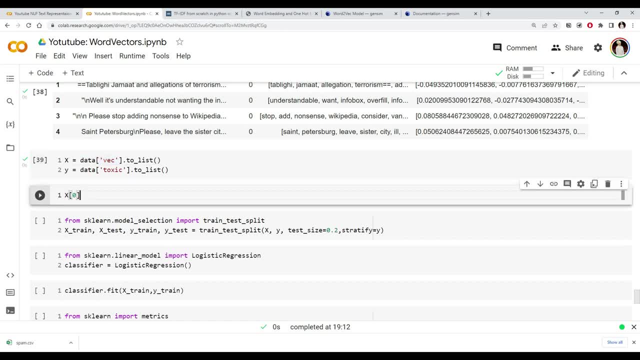 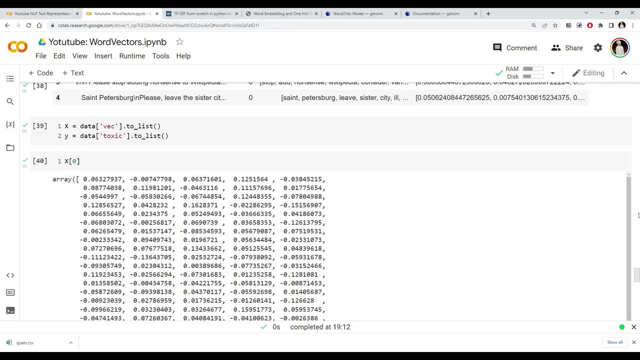 that column and convert it into the list format and you can see: x is our training data, y, we can think of our labels. and let's look at the first example. so nothing but the vector that we just saw. this is the 300 dimensional vector. what we have. 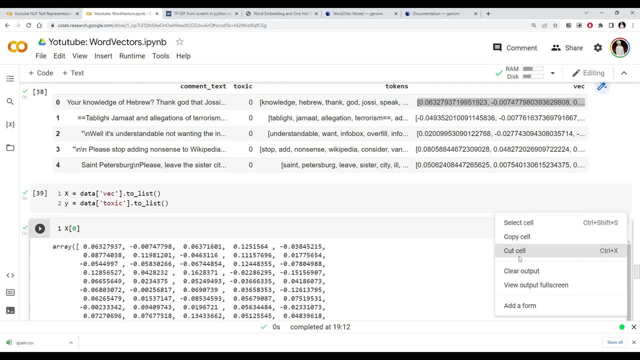 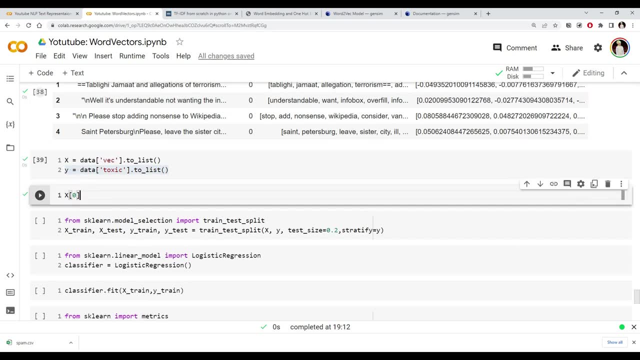 okay, that we're going to pass to a machine learning model for the classification. and then you have here toxic, which is nothing but the zero and one. all these things right again, we will use the train test split from a scikit-learn and, you know, split our data set x and y into the 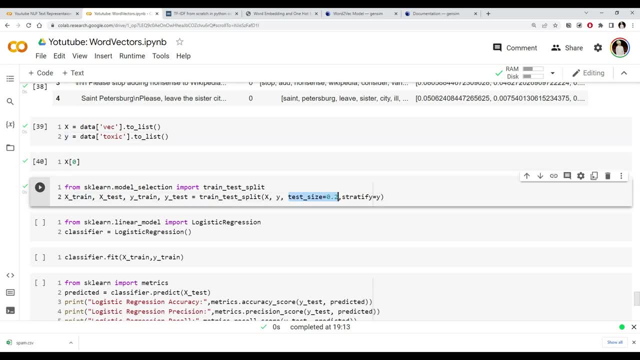 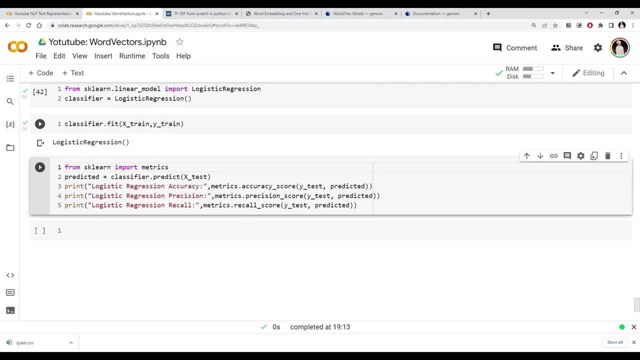 training and testing. making test set as a 20- i'm using some basic model like logistic regression from the scikit-learn- and then fit our training data, which is x train and the y train, and once we fit our data, let's predict on our test data and see the accuracy. 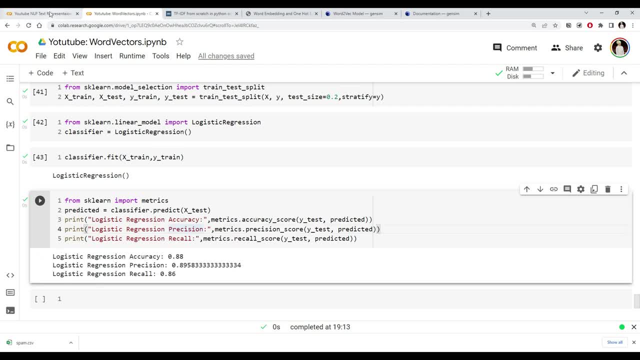 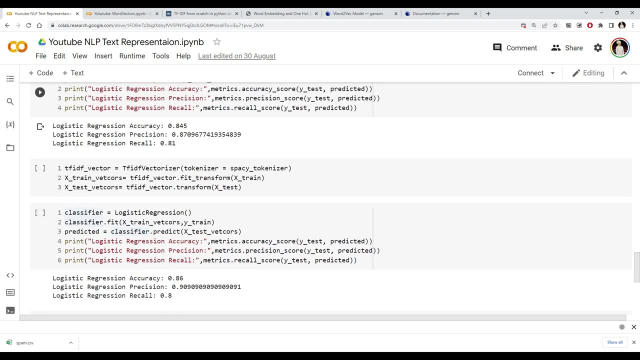 and we got some, you know, here let's compare with what we had got with the tf, idf and the thing right. so this was the tfi. uh, this was the count vector. this is the tf idea. look at this thing for accuracy. we got 88 percent here we had 86 percent. here we have 84 percent. so 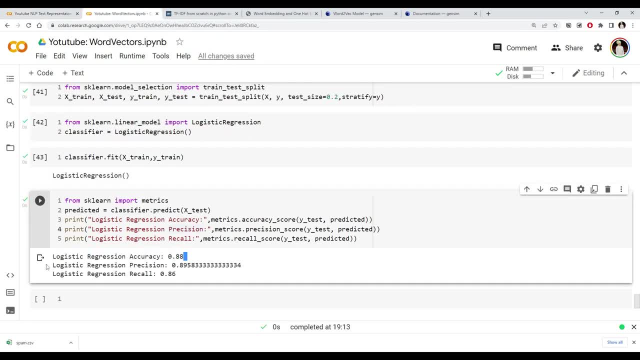 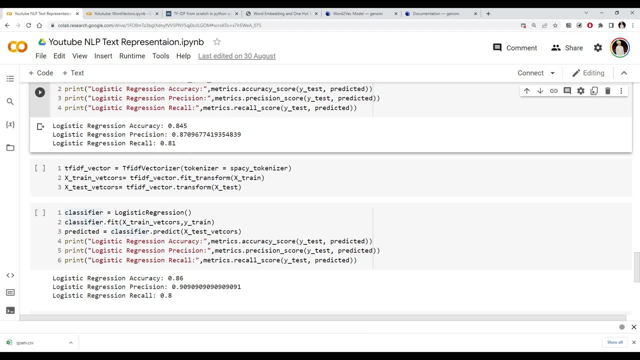 it seems to be accuracy got improved, using our word to wake representation. what about the precision? here it is 0.89, here we have 87. here we have nine zero. so if you look at the precision we got, you know less precision compared to what we got in the tfidf. actually slightly less. what. 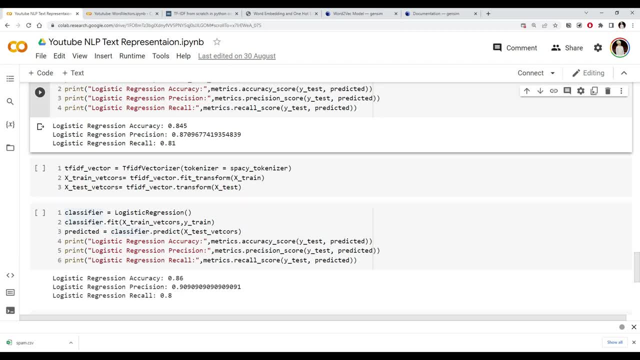 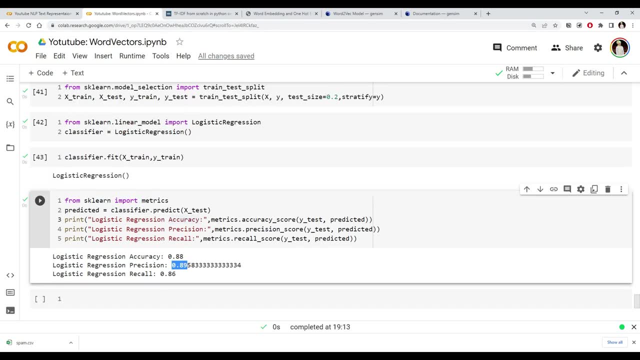 about the recall. recall there is a significant improvement. you can see where we have 0.81, here we have 0.8, but here we could see we have 0.86, which is pretty significant improvement what we got on the recall. so i think this was the um. so if you look at the overall, you know metric, we can say: 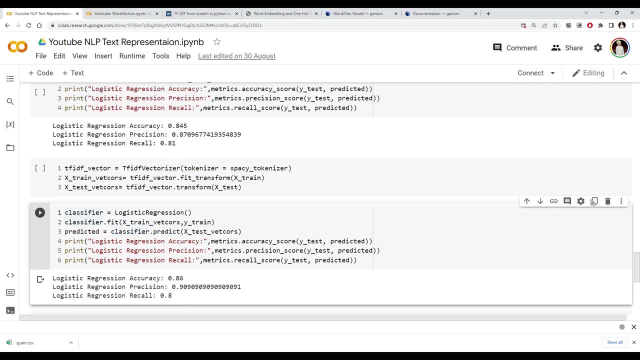 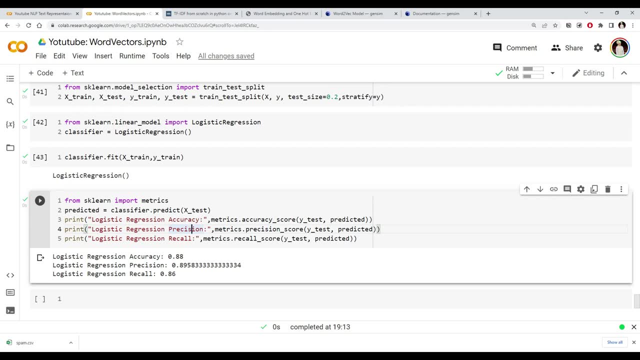 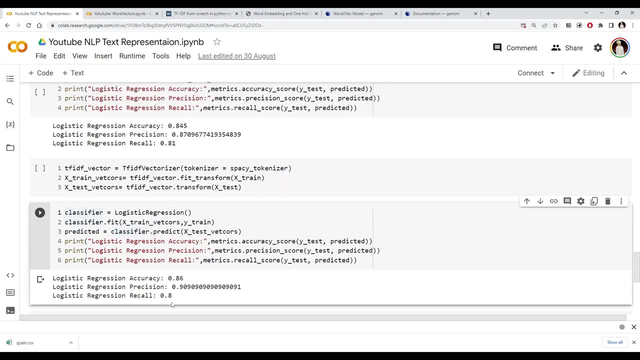 that word to wake is working better than the tf idf, and this need not to be case, though theoretically we know that. you know that word to wake should work better compared to what we have, tf id. but you should always do an experiment. you should at least check what you know, accuracy or the metric. 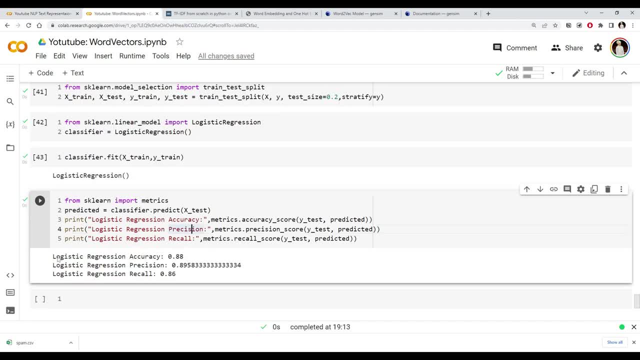 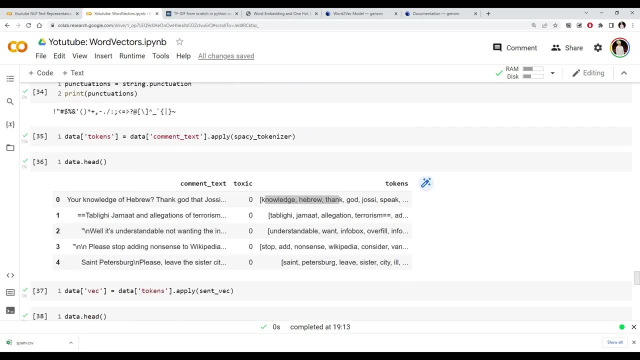 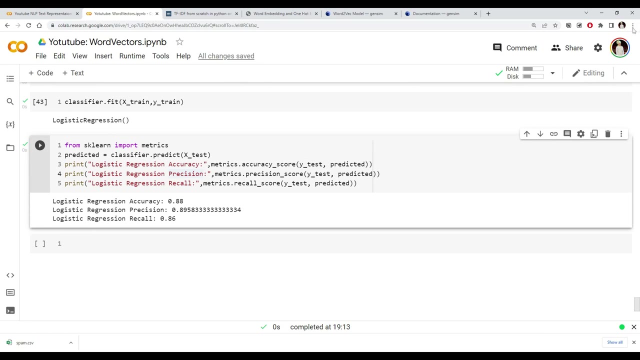 you got on tf, idf and what you are getting with the word vectors, right. so this is what. this is how you can. you use the pre-trained word vectors and feed that particular word vectors to the classification model and and do the classification. and i couldn't spend much time on the theory part. 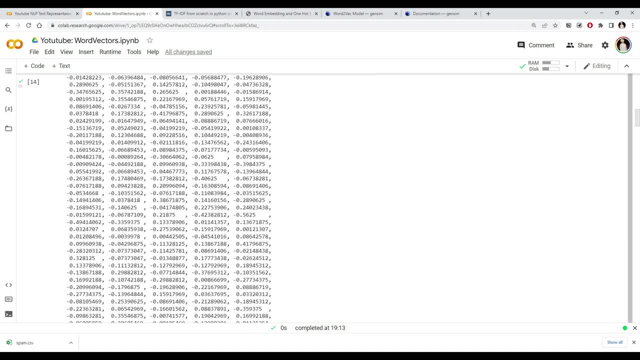 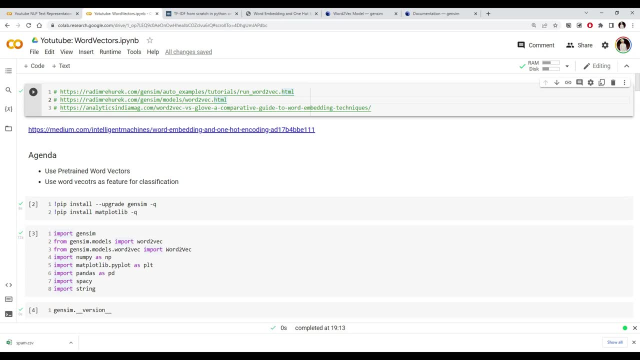 of it. but i would suggest go and, you know, read about uh this particular you know word vectors. how, how do we, we exactly train those word to wake models? right, whether it's a neural network or what kind of algorithm it is, and right, so you can read more uh about it and do some hands-on with respect to this part, you know. 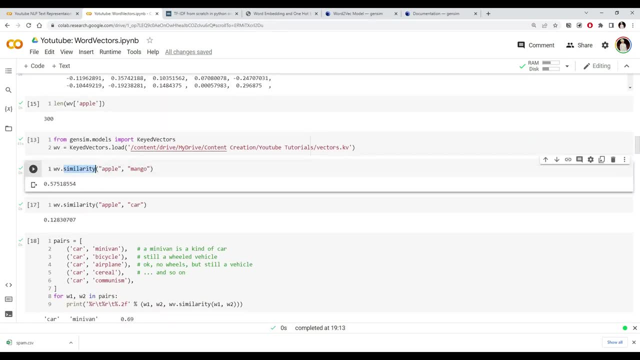 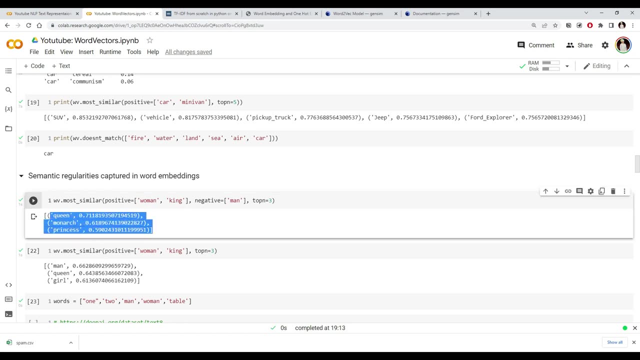 you can create some simple application using this thing right, checking the similarity between the words and, you know, finding on which word doesn't match. so these are the good thing. so we can even train our own word to wake model. so if you look at the- uh, you know- documentation of jane sim you. 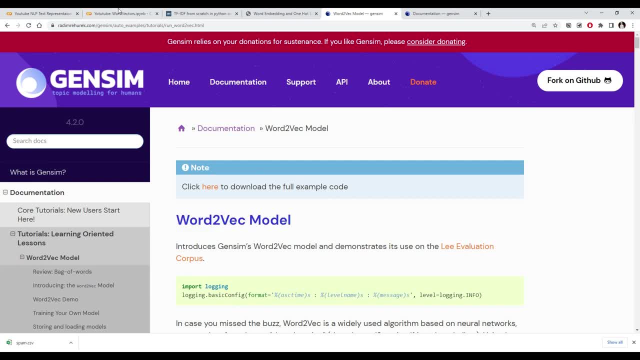 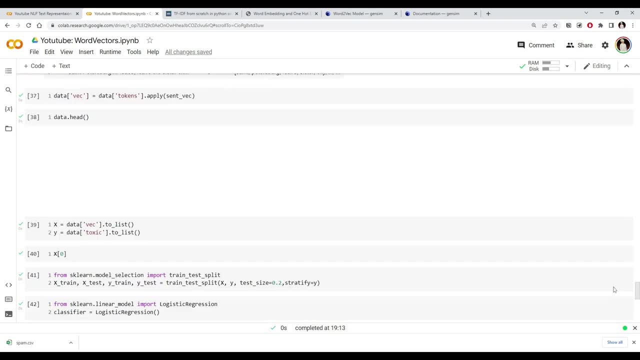 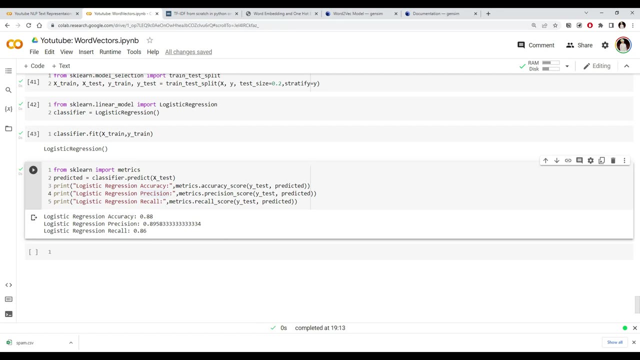 will see how to train your own what to wake model. currently, we have used pre-trained model, which is from the google, but you can also train your own word to wake model and then check whether the accuracy of your pre-trained model and compare it with the your own train what to wake model. maybe i 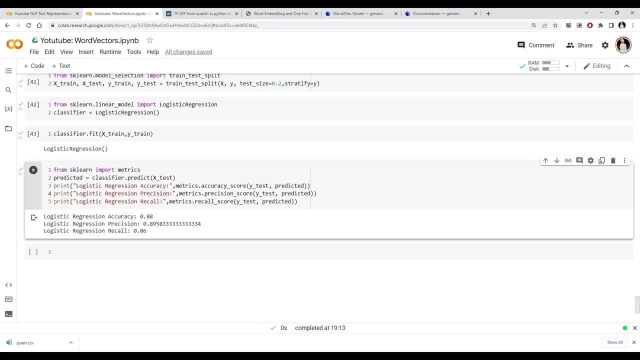 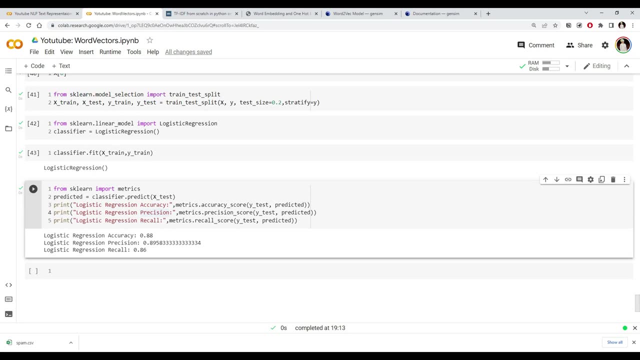 can you know next video i might do on that? uh, not sure, but you guys can do that and i will see you in the next video. bye, bye. can uh do an- you know experiment with it and let me know in comments, you know, what observation you find. you can try different data set and do you find that what to make is? 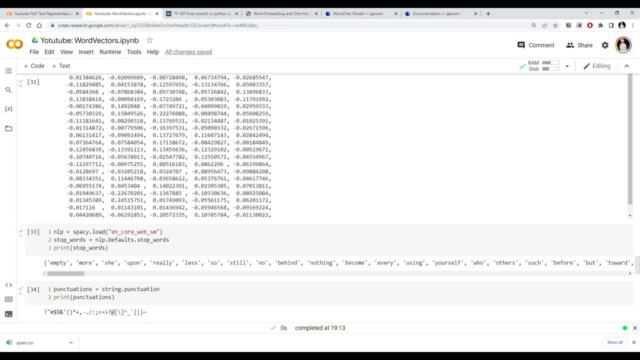 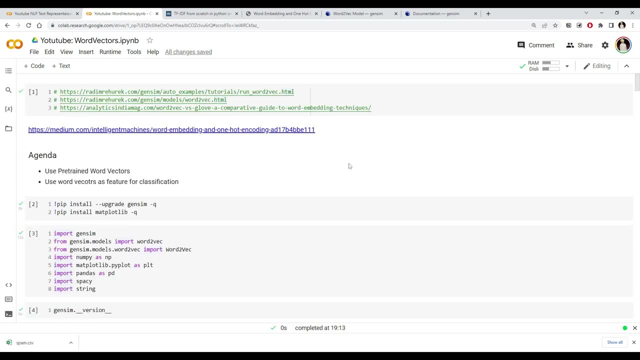 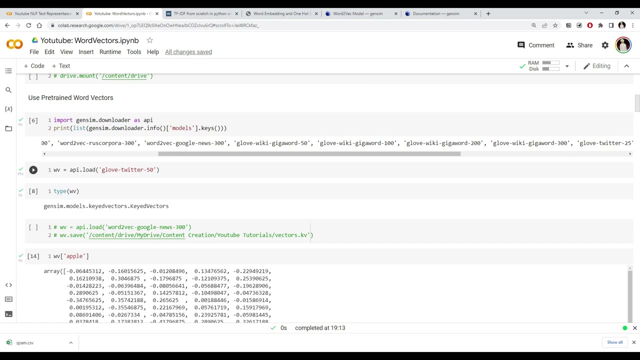 always better than pfidf, or that is not the case, right? so you can do all this thing later. so thanks for watching. i hope you found this video useful and i will be sharing this code so that you can do your. you know hands-on with this particular thing and if you haven't subscribed to my channel, 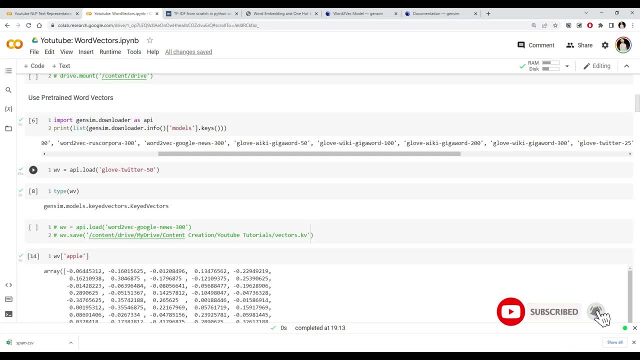 please do subscribe. i saw recently we have crossed like thousand subscriber. that is definitely motivating and i will be creating, you know, more natural language processing video. thank you,